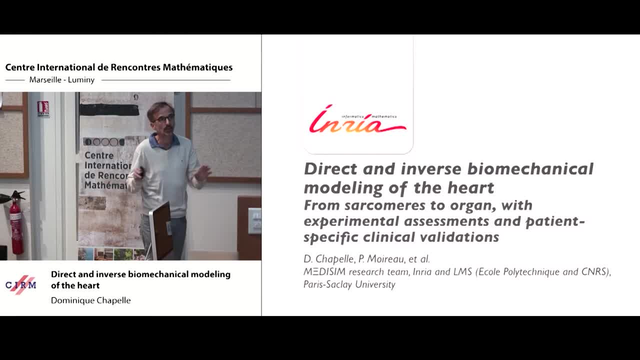 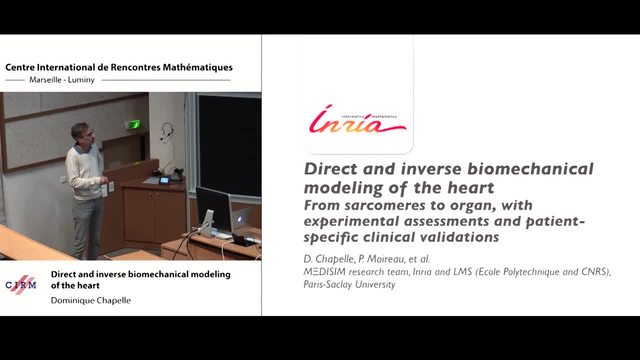 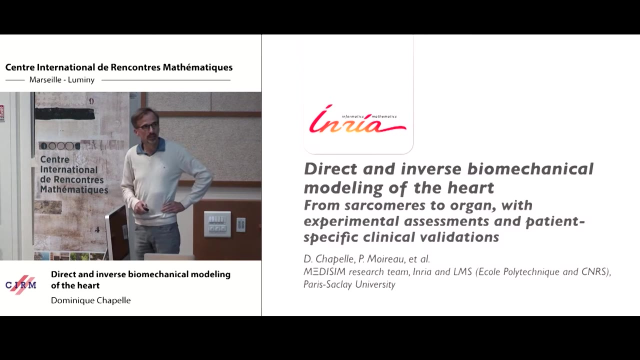 this will cover quite a wide area of subjects. that is going from multiscale modeling to experimental validation and clinical applications, with a specific subject That will be patient-specific modeling that I will tell you about soon. So this is really teamwork that I'm going to present Medisim, that is an INRIA team. 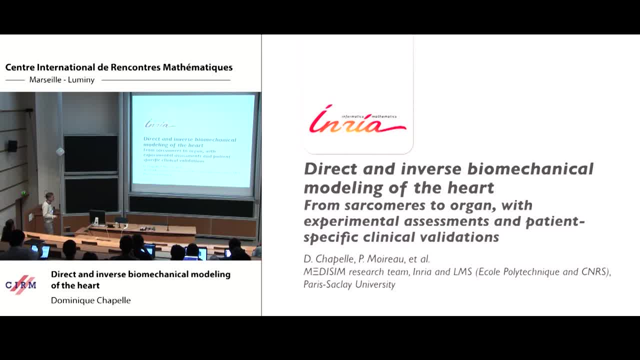 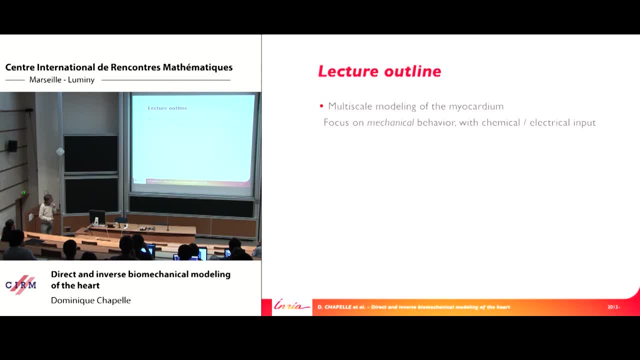 now joined with LMS, Laboratoire de Mécanique des Solides, Ecole, Polytechnique and CNRS, The outline of my talk. So again, this will be biomechanical modeling and vastly multiscale, as you will see in a minute. 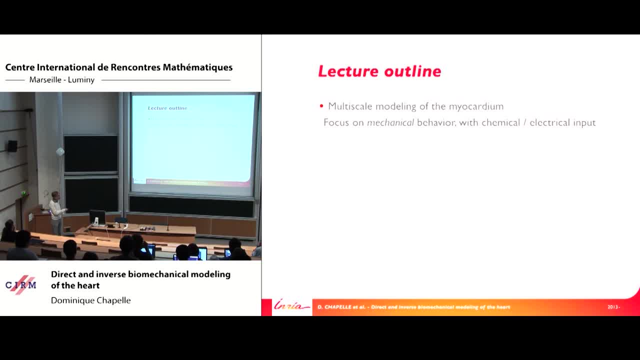 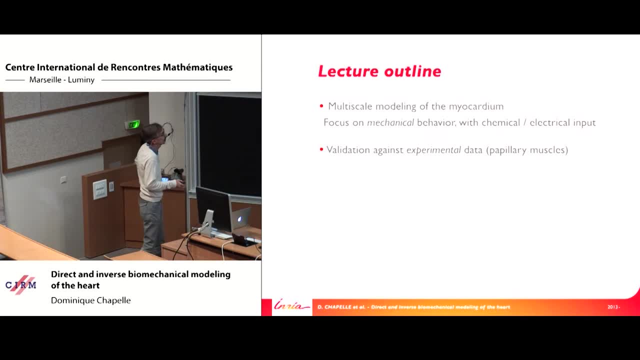 So focus on Mechanical modeling, and the electrical, chemical input phenomena will be seen as an input to the mechanics. We'll cover some validation using experimental data, you will see. and now, of course, we need to not only talk about material modeling, but also organ and system modeling, and this 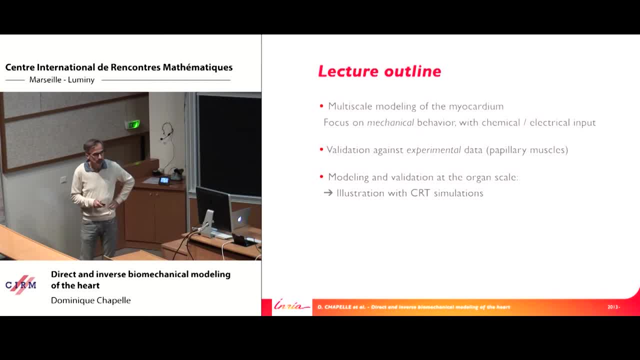 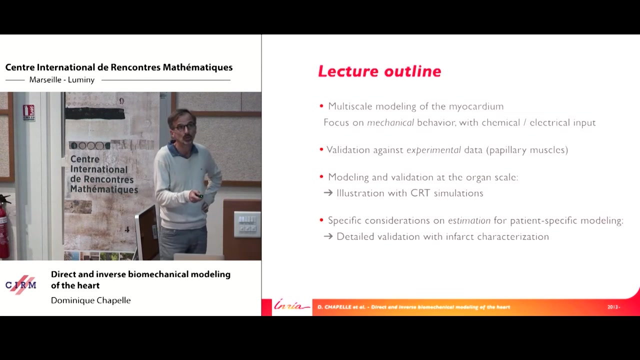 will be illustrated with A clinical application that's called cardiac resynchronization therapy, CRT, and the last part of my talk will be dedicated to specific considerations regarding inverse problems aimed at estimating the model for the purpose of patient-specific modeling, so adapting the model to a given situation, and again with a detailed validation. 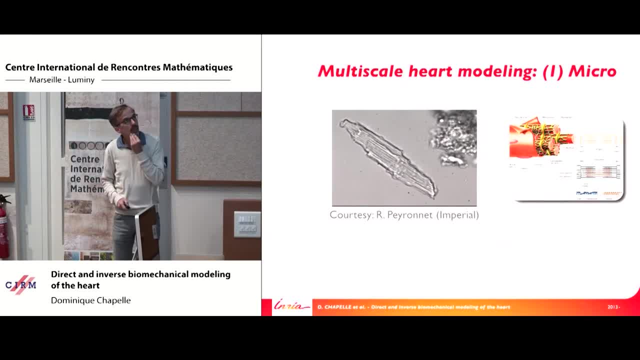 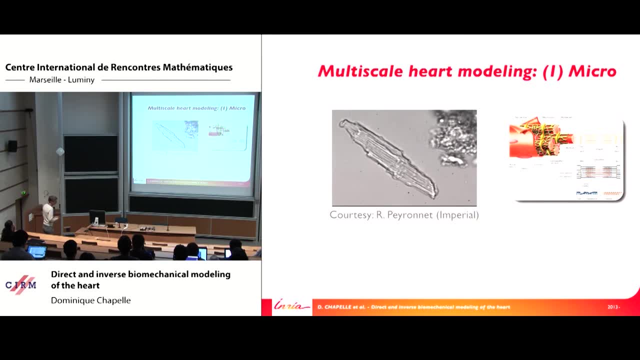 Modeling of the heart starts, of course, from the myocardium. that is the material itself, the muscle that we need to model and, as I mentioned, this is hugely multiscale because it starts actually at this scale and below. This is a single myocyte cardiac cell. 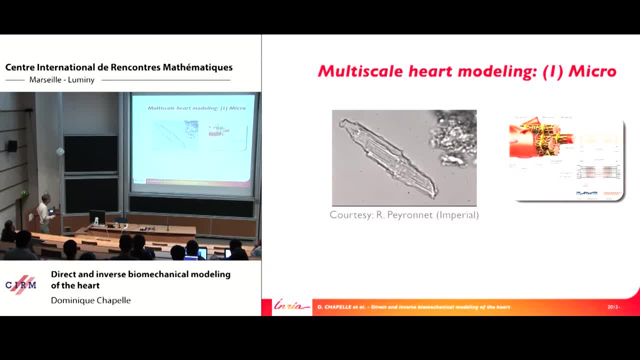 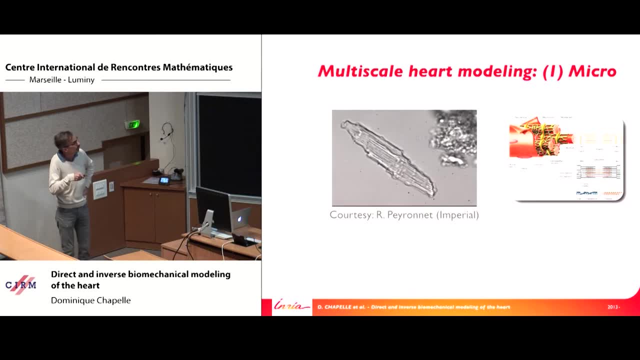 Okay, That is beating live, so to speak, in a microscope. This is typically 100 microns long here, and below this scale. the bending structure that you see here translates reflects the basic entity of muscle contraction that lies within the cells and that's called the sarcomere that you see here. 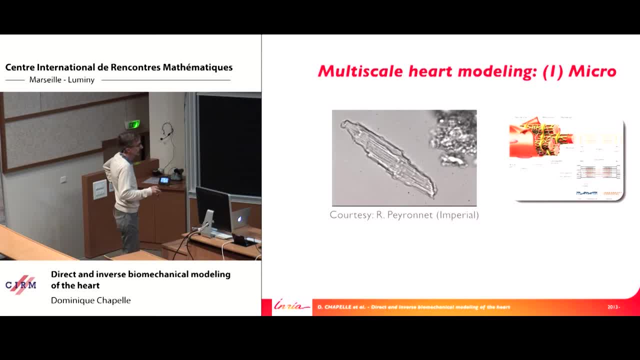 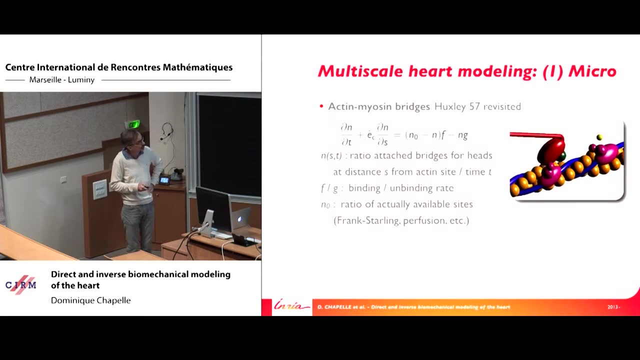 So two bands. They denote the ending of the sarcomere, and the sarcomere is made of a specific arrangement of two types of filaments, so-called actin and myosin filaments that are able to create bonds with each other. 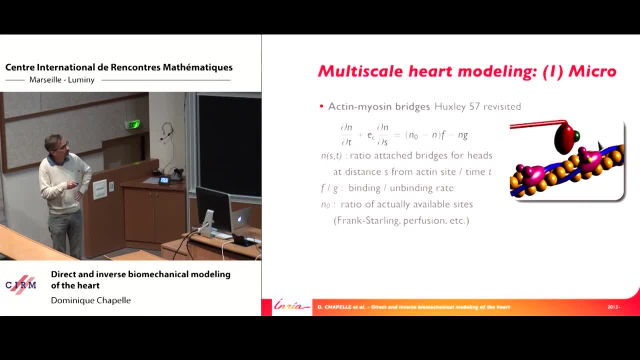 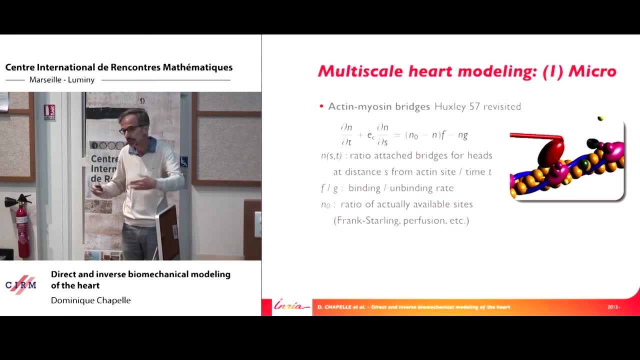 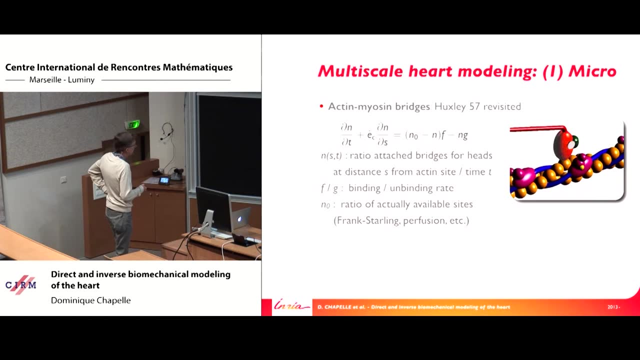 So there are head-like structures on the myosin filaments that can attach on the other actin filaments and that creates forces that tend to shorten the whole structure. The basic type of description that we use is actually inspired from Huxley, who was 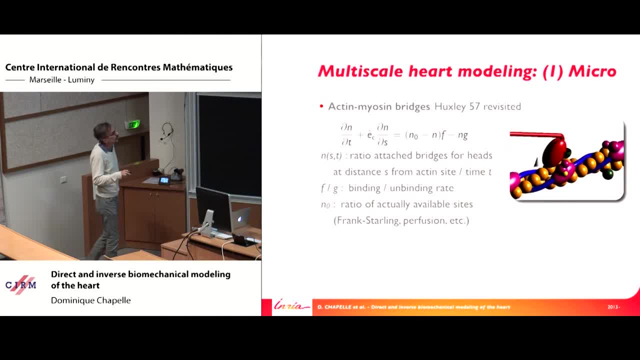 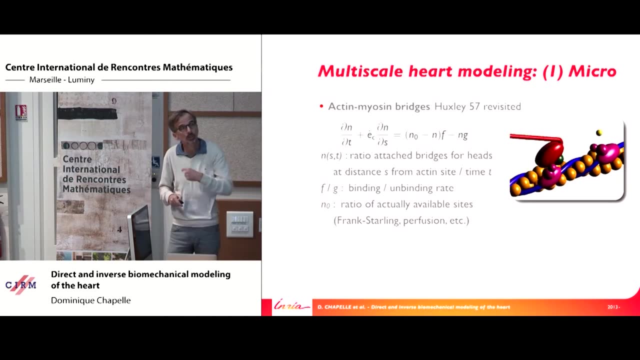 a great man in cardiac modeling. So we've revisited a model that he proposed in 1957 to describe, statistically speaking, the attachment of such heads, so-called cross-bridges between heads, Cross-bridges between the two types of filaments, via the n- quantity that's here and n denotes. 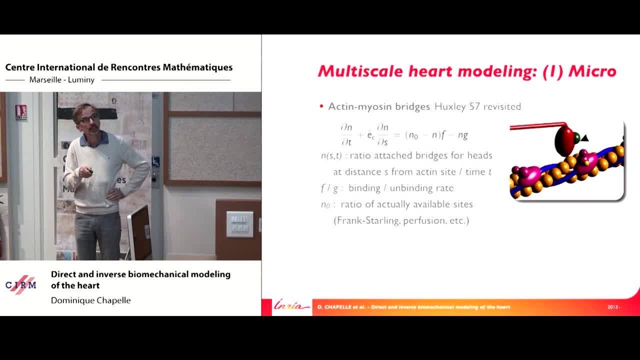 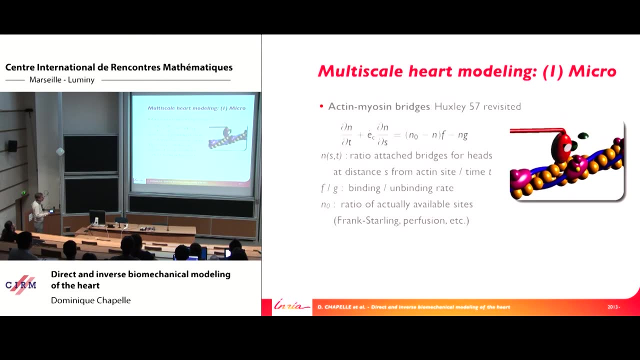 for the population of heads that are located at the distance s from the nearest actin site at a given time: t So for this population, the ratio of actually created bridges. So this is really accounting for these myosin heads. That is the difference. 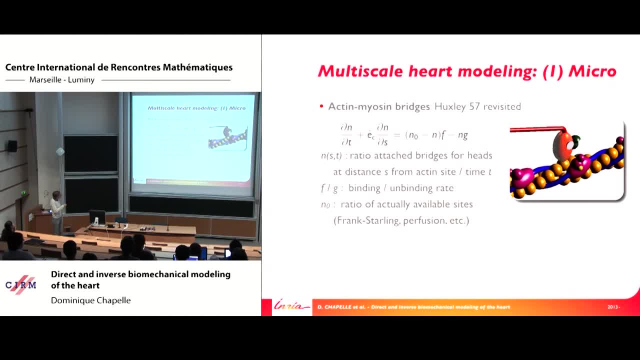 It's described by this equation. So what we have here, EC dot, is the strain rate, extension rate of the whole sarcomere. So the filaments slide along each other. This is the so-called sliding filament theory. And in the right-hand side what you have is creation and destruction rates F and G. 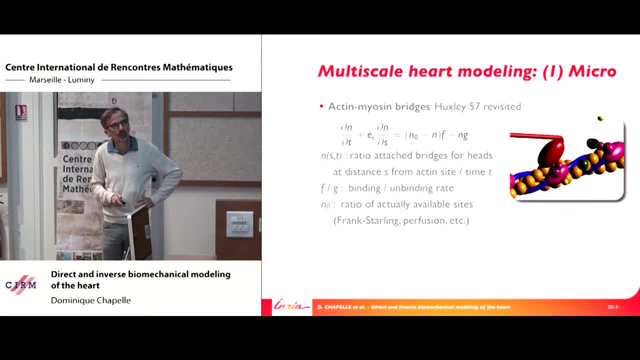 And n zero would be another quantity. Okay, Okay, Another function to model So essentially here to obtain So. s again denotes the. It's important as a variable in this equation, other than the time, S is the location, the distance to the nearest actin site. so that would be the extension. 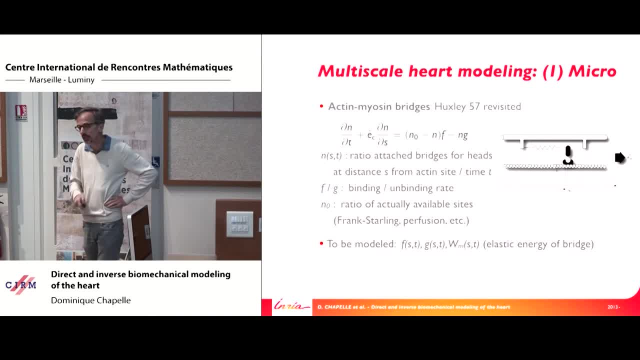 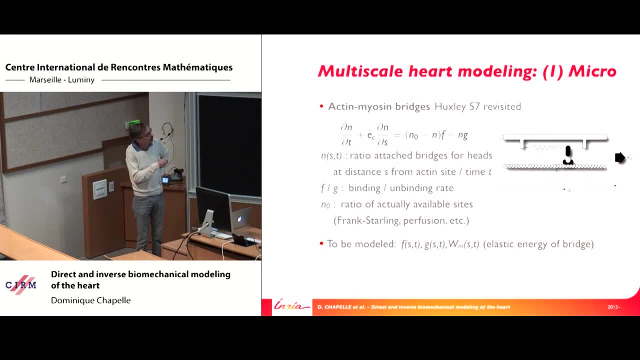 of the myosin head if you represent it like this, like a spring-like structure when the head is actually attached. So here what you need to model to in a way, close the whole problem are the creation and destruction rates in the right-hand side and the energy that would be created in a 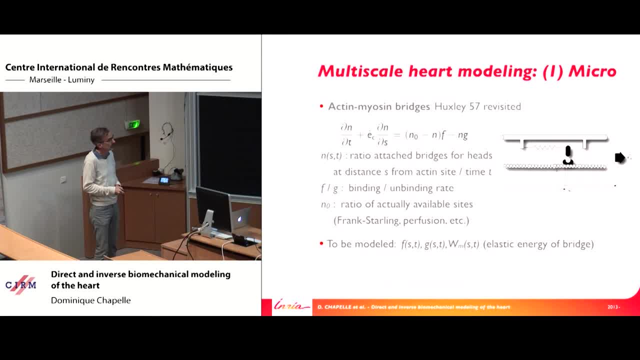 cross bridge. once the bond is actually created And once you have modeled the energy, in particular with the n variable, you can average over the whole population to obtain. So this would be d. The derivative of d is the derivative of d. 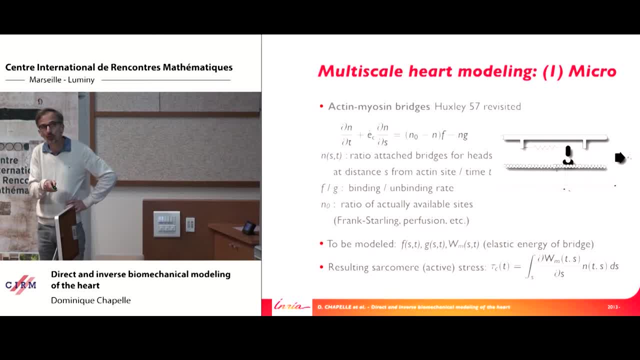 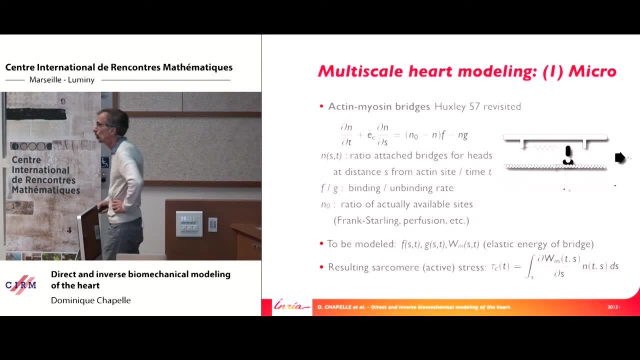 Okay, So the energy with respect to extension would be, of course, the force created in a single bridge. So if you average over the whole population, using n, you obtain the total force, the average force created in a sarcomere. 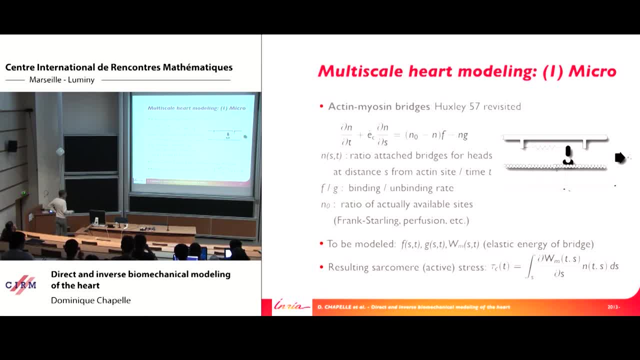 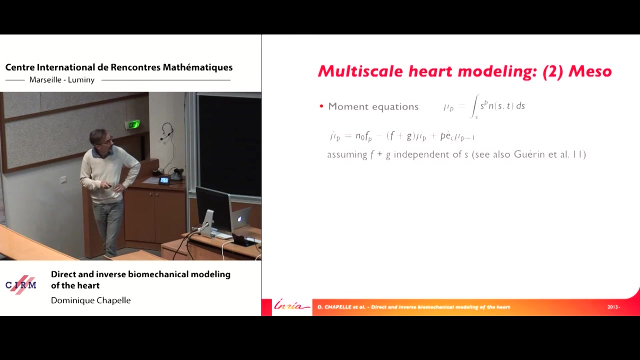 So this is how we will travel over the scales using the n variable. More generally speaking, a type of equation that we can look at pertains to what is called the moments of n. So moments are obtained, Okay, by weighing powers of s with n over all possible values of s. 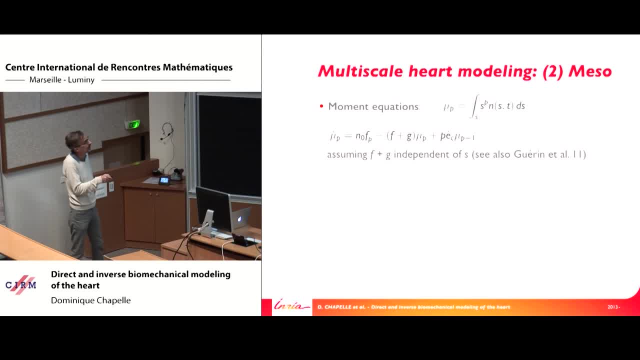 And if you multiply the Huxley equation by s to the p and integrate, you obtain a dynamical equation like this: on the moment of order p, that relates the variation rate of mu p to the previous moment and, of course, quantities that are inherited from the rates. 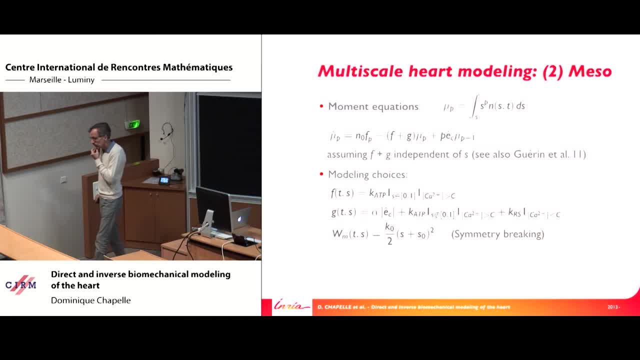 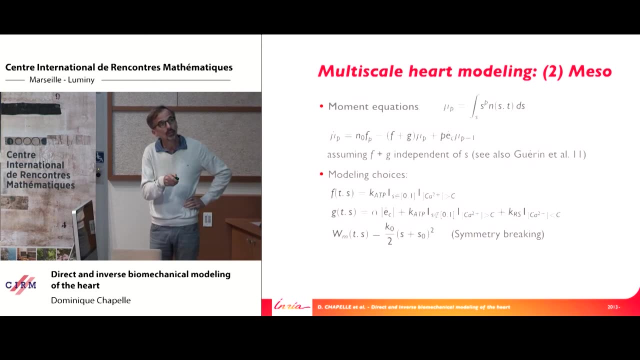 Now, what we frequently consider in our models are the simplest modeling choices for the three quantities that I pointed out on the previous slides. So creation destruction rates: essentially two different chemical reaction rates depending on a switch that represents the calcium concentration above or below a certain level. 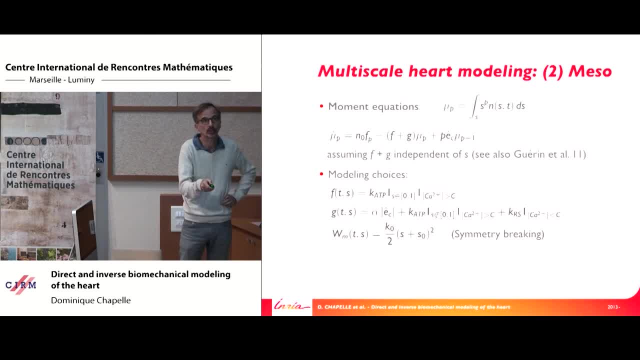 So if you look at the, Okay, If it's above, you create, If it's below, you destroy the bonds. And for the energy of bridges, the simplest you can think of is, of course, quadratic energy, with a little shift. 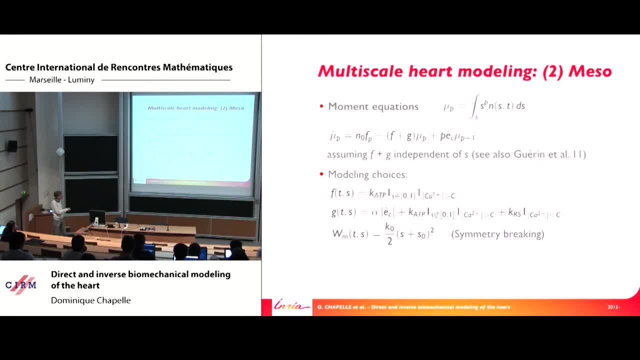 That means that when you attach you're already under tension. So this is so-called symmetry breaking in physics. This is described in more details in various papers, But again, these are the simplest choices that you can think of. And now at the macroscopic level. so if you consider the average, the integral of n. 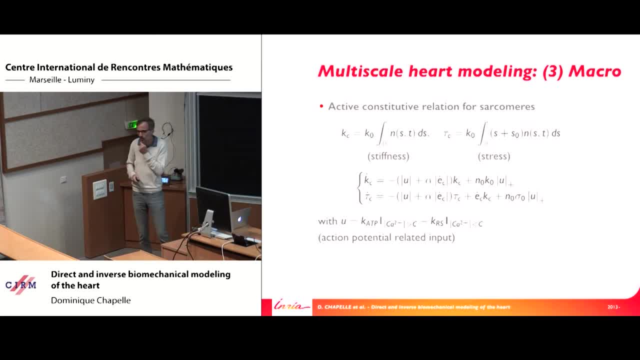 you will obtain something that's proportional to the total number of actually created bridges at a given time- t. So the kc here only depends on t. of course It's average over s. So if you multiply by the individual stiffness of one single bridge, you obtain something. 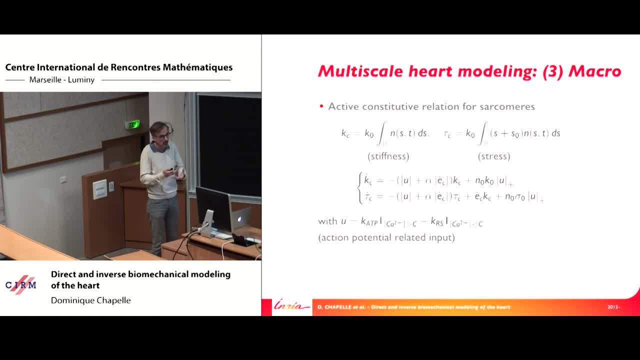 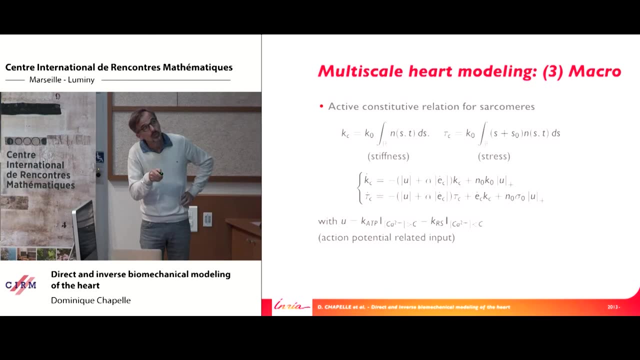 that denotes that represents the stiffness of the whole sarcomere. So this is the moment of order zero. on the previous slide It's the integral of n multiplied by s to the zero. Now the stress created in sarcomeres. again, I showed this on the first slide. 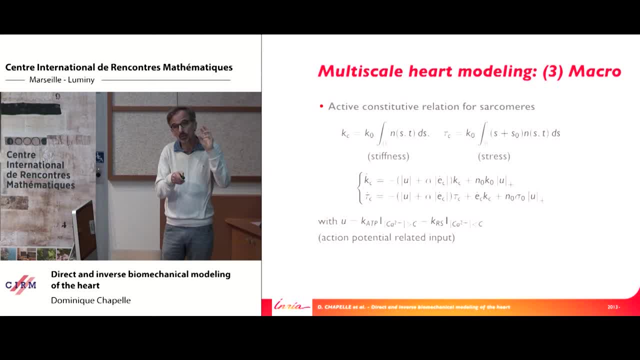 The first slide would be obtained by differentiating the energy of a bridge. So this is this quantity here And you can see that it's a combination of two moments: zero order and first order moments. Now, if you write the equation obtained from the moment equation on the previous slide, 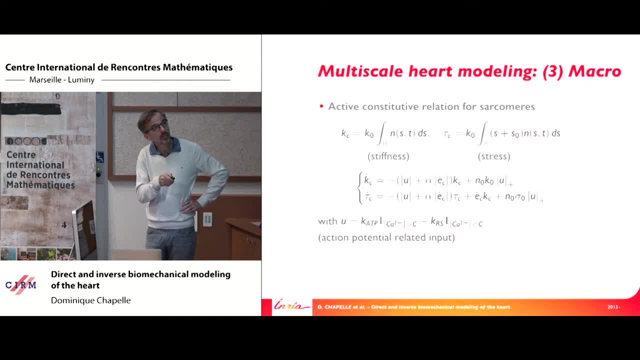 you obtain these differential equations here, this ODE system here, that describe tau, c, the stress in a sarcomere, and kc, the equivalent stiffness of the sarcomeres, And this you can think of as some kind of complex constitutive equation that relates 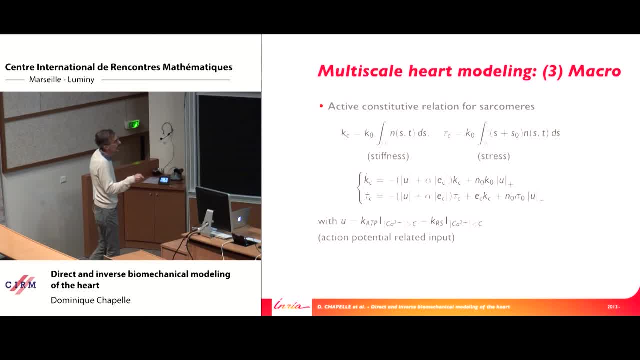 the extension strain to the stress via, of course, some time-dependent equations. So the rates are appearing here And the system also needs The system also needs this equivalent stiffness as an intermediate variable. And u here is directly something that is inherited from the rates, the chemical rates. 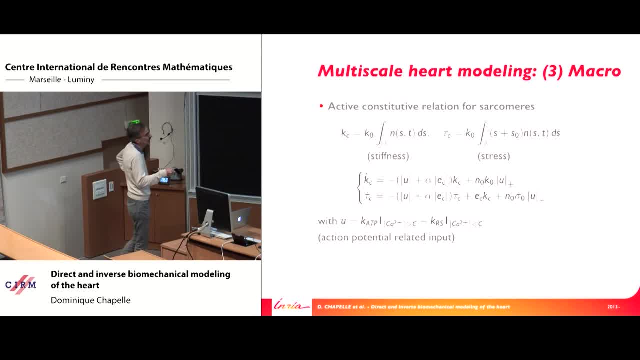 that appeared on the previous slide, So it's a summary of f and g if you like. So u is one constant if the concentration is above the threshold and minus the other one if it's below. But likewise you can also monitor the microstotic energy, that is, the energy that is stored. 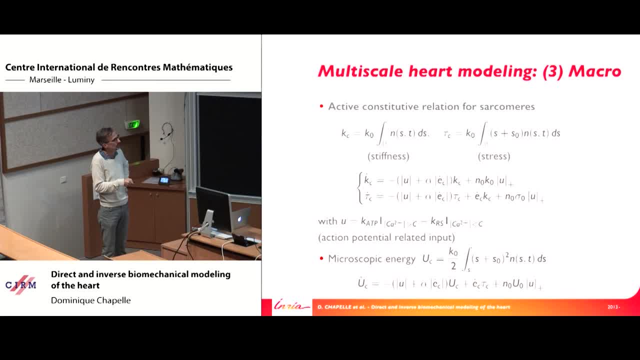 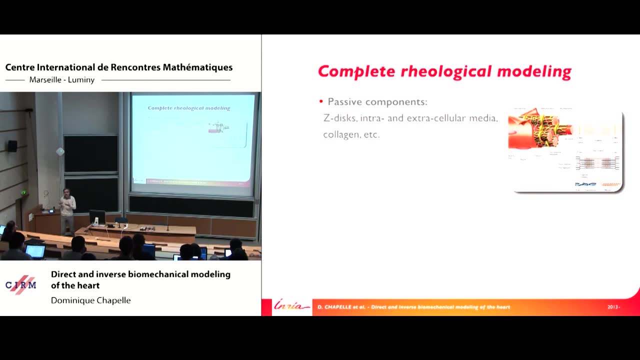 within the chemical bonds, And this would use the second-order moments in addition to the first two, So you can obtain an equation that describes the energy as well. Now, this was for the active behavior, so the active forces that are created within the sarcomeres. 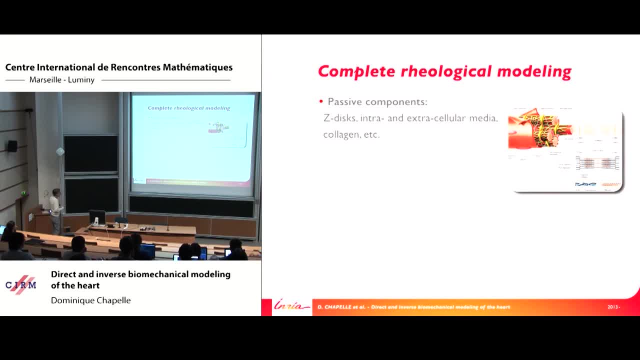 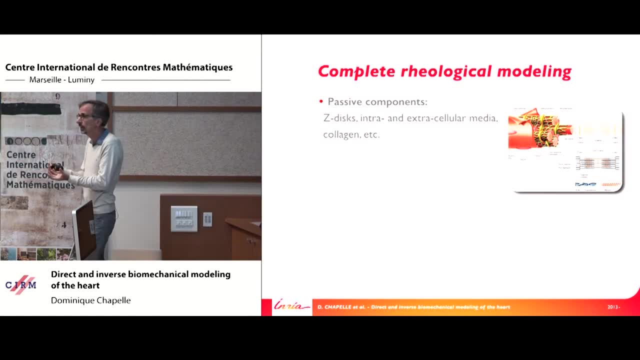 Of course it's not the whole story, because there's a lot of passive factors, But this is what we have here. OK, Good behavior also in such a system, in particular for the endings of the sarcomeres and then for the whole cellular envelope and beyond for the extracellular matrix. so all this. 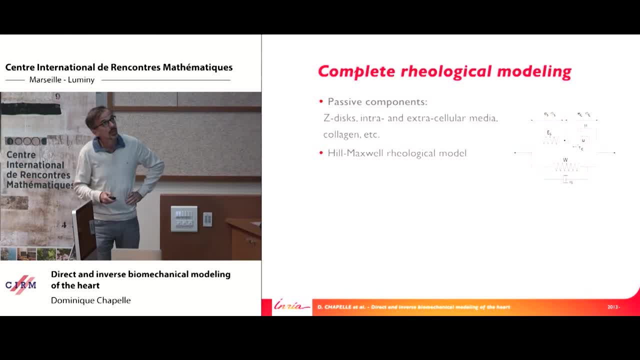 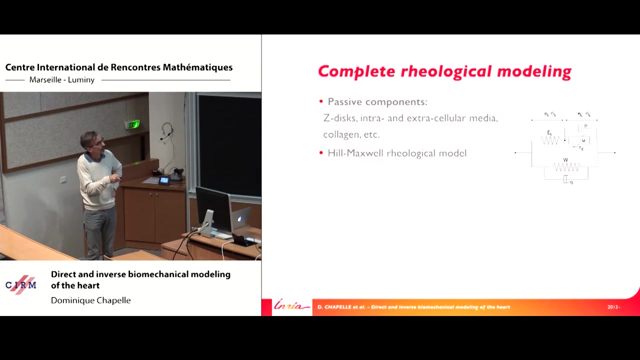 need needs to take to be taken into account, and this we do by rheological modeling, in which various types of behaviors are aggregated within this type of spring combination and dampers combination analogy. so here the sarcomeres would be at this location over here, and it's in series with some elastic components in parallel with. 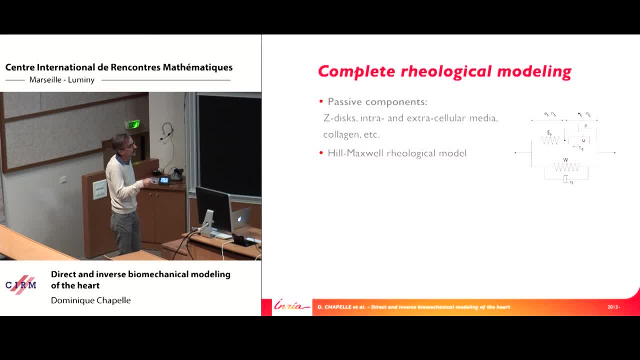 viscosity. this is quite typical and then so this would be the end endings of the sarcomeres, typically, and then in parallel with, again, viscoelastic behavior for the cell envelope and the extracellular matrix. What's important is that the sarcomeres essentially create forces and stresses in the direction. 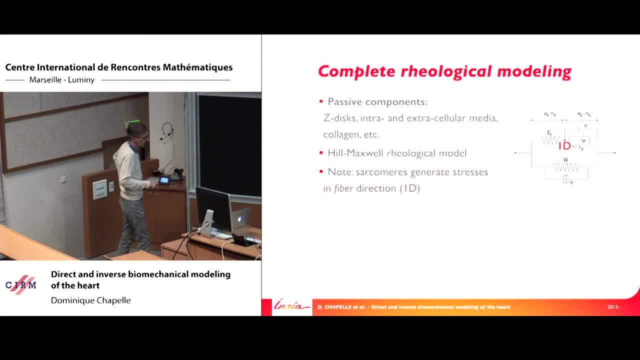 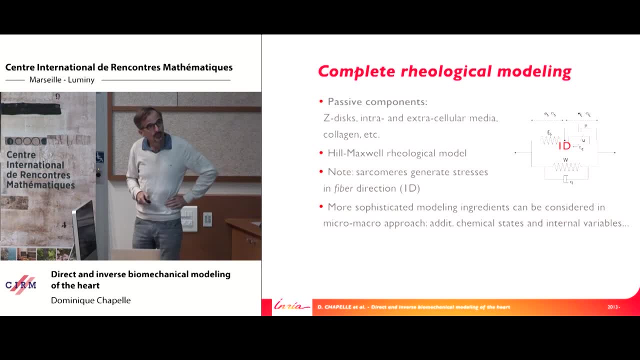 of the muscle fiber. This is essentially 1D, what you have in the top branch, and the rest is, of course, 3D. This is one way of modeling, but of course you can sophisticate as much as you like. 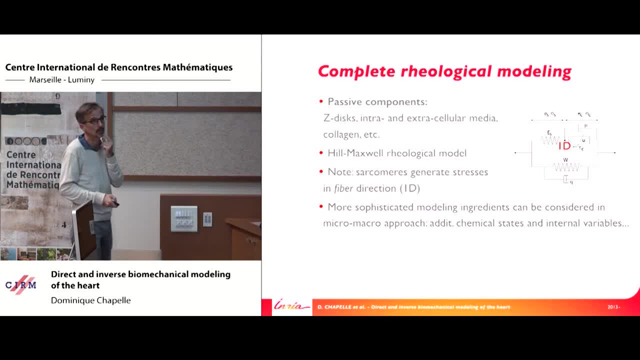 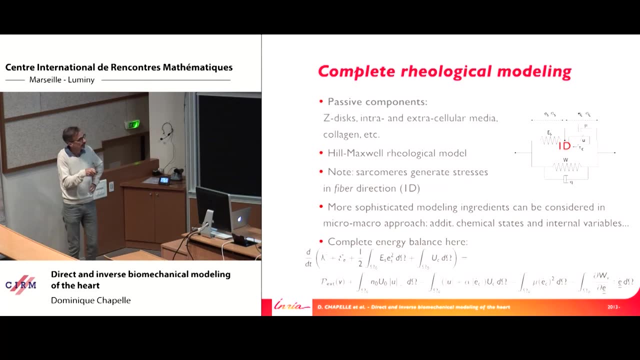 starting actually with the description of the sarcomeres themselves. so we could take additional chemical states- Here you had only two for the myosin heads and additional internal variables. Okay, Now this schematic here I mentioned it was an analogy with springs and dampers. 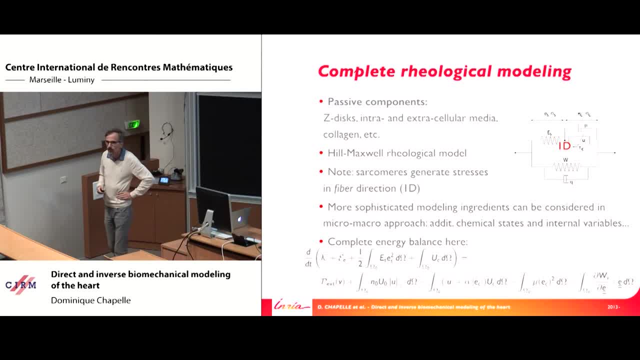 It needs to be interpreted in a consistently nonlinear manner, because the strains that we're going to look at are large, so not only displacements but also strains are large. This needs to be revisited in this framework if you want to be energy consistent, which 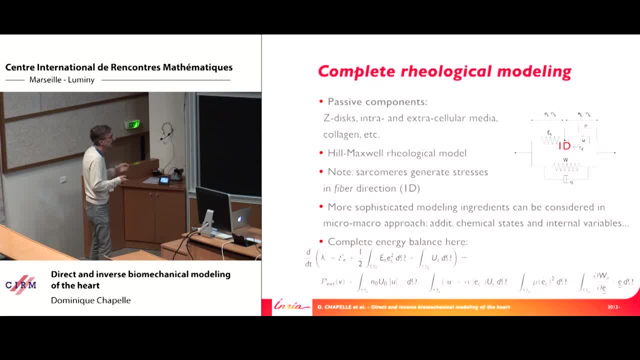 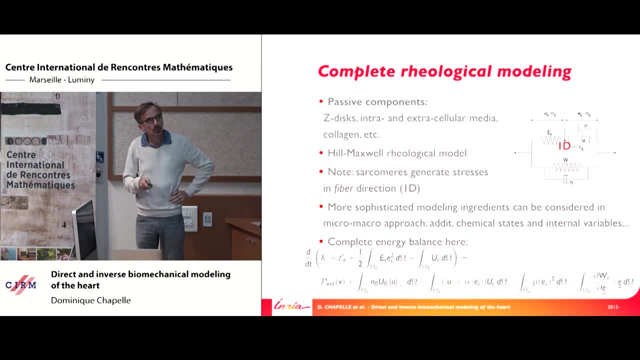 is essential here, like we heard yesterday. Okay, In climate modeling. Once you do this, you can obtain the complete energy balance that describes the variation of the total energy, so kinetic, elastic stored here and there, and then the elastic energy stored in the sarcomeres, with external power of forces. 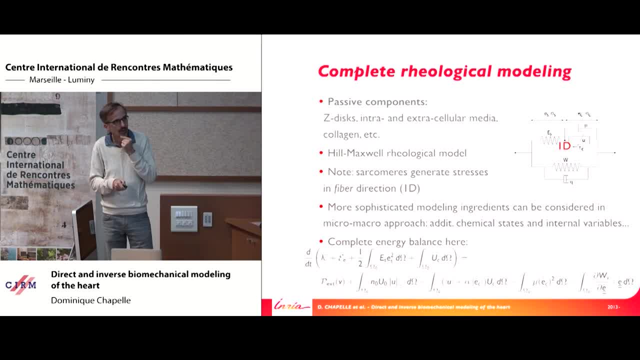 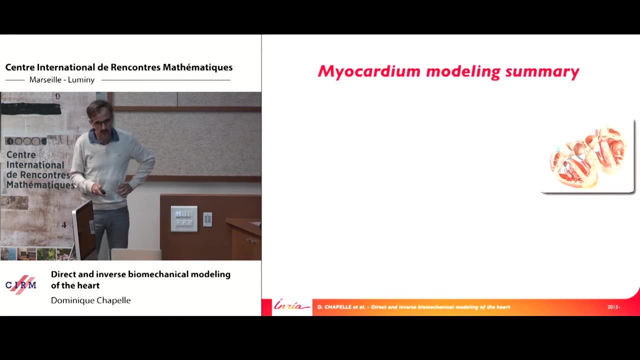 This would be the engine inputs, due to So, the positive inputs. due to So, the positive inputs due to chemistry, and these are dissipations. Some more details quickly regarding the whole behavior. so the fundamental equation would be the principle of dynamics, the so-called principle of virtual work. that's written. 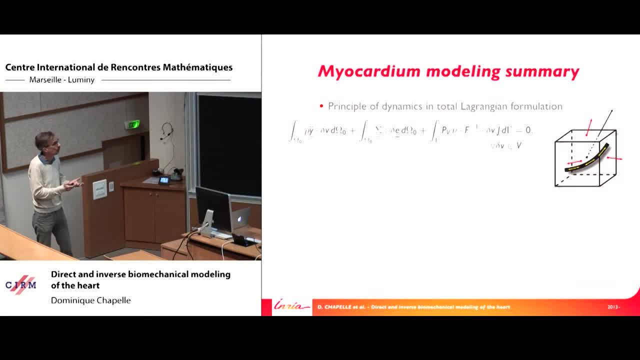 here in total Lagrangian. That is, you use a reference configuration to describe the displacements, So y double dot would be the acceleration. Here you have the inertia effects. Here you have the external forces, represented here by, essentially, pressure, against which? 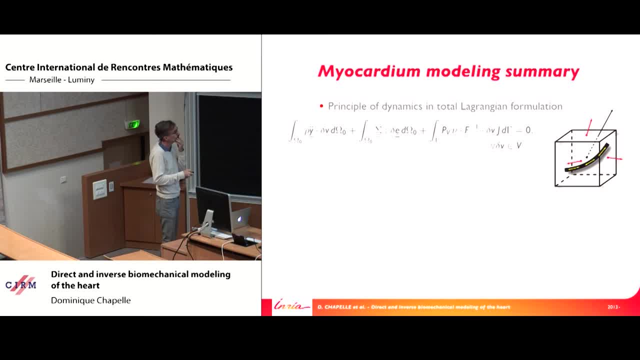 the heart walls would actually work. so external loading: Here this is the internal work. So here this is the internal stress tensor that you have in capital sigma And capital sigma aggregates the various components that I described on the previous slide. So that is, we'll take hyper-elastic parts, viscous parts and the part that was in the 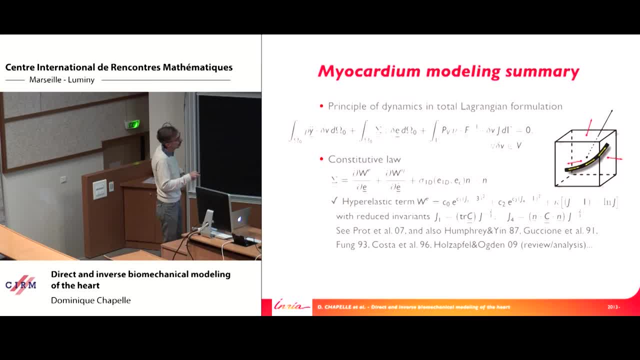 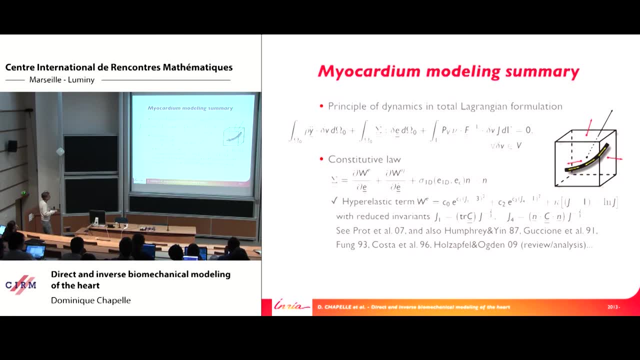 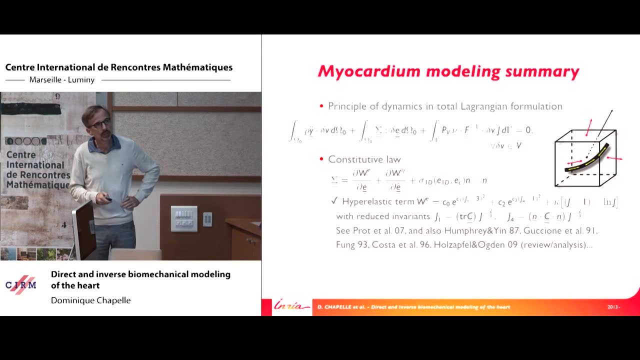 1D sarcomere branch For the hyper-elastic term. we use something that's very standard in biomechanical modeling, that is, exponential laws, plus something that allows to model incompressibility- Okay, Because biological tissues are frequently very incompressible- say. 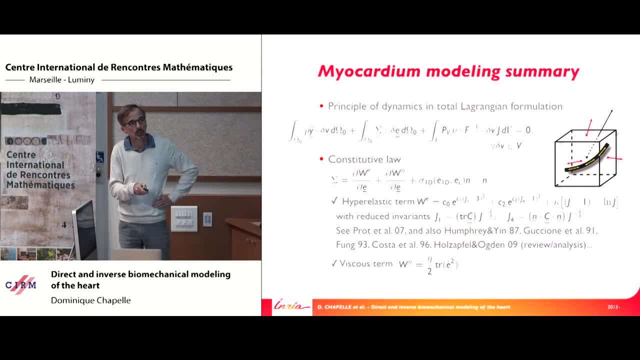 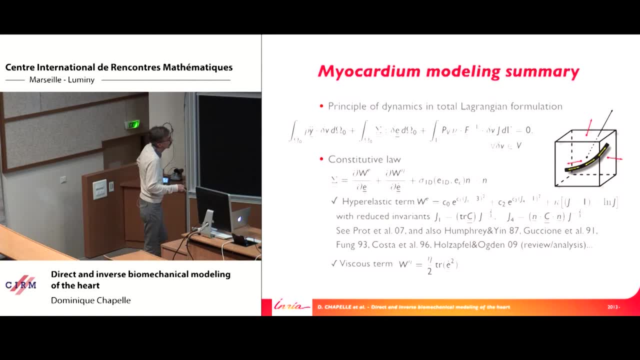 Another viscous term that's. here we take the simplest that we can think of, so something that's essentially the square of the strain rate And again the active parts that will govern this 1D stress tensor along. This is the fiber direction N. 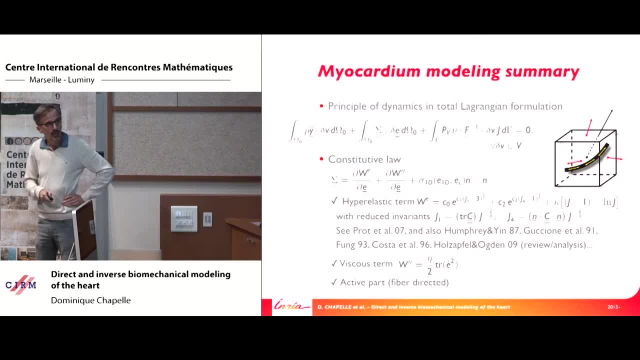 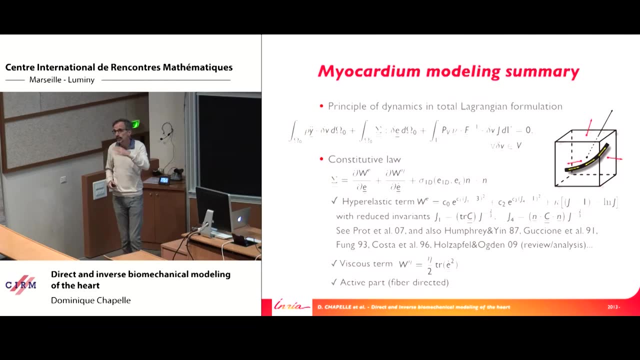 So this gives you The second order tensor, And this stress tensor, directed along the fiber direction, is the result of the sarcomere modeling. So this is a very fast overview of the type of modeling that you can perform, But now we have something that's complete, that's quite general, because this is one 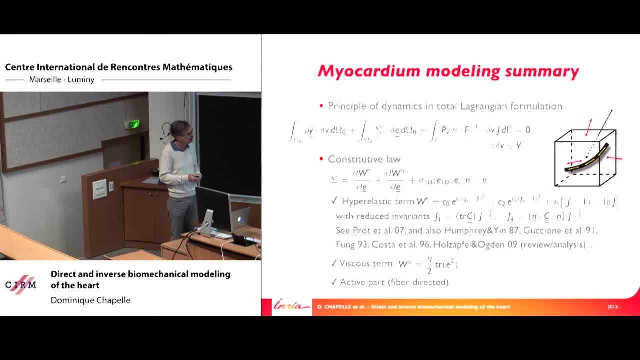 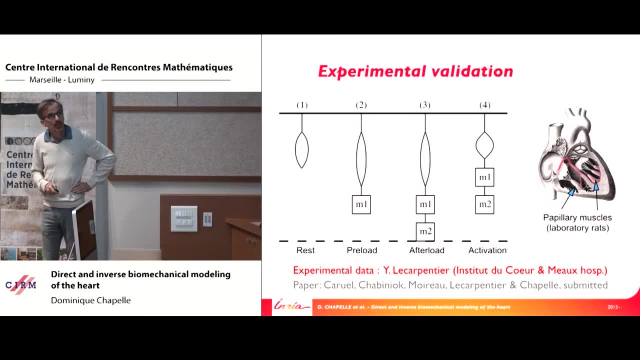 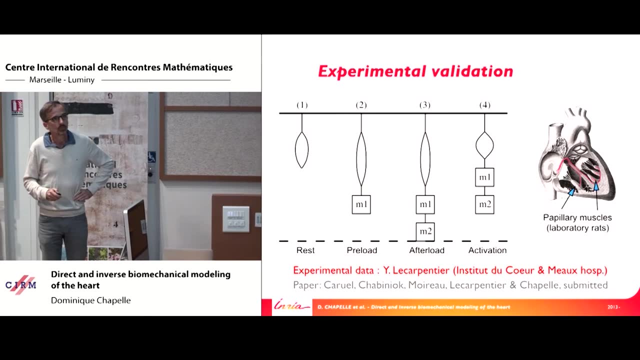 choice, But you could use other considerations. Okay, You could use alternative choices And that's again energy consistent. Now let's look at some experimental validations that we performed for this model. So this is at, I could say, at the local scale. 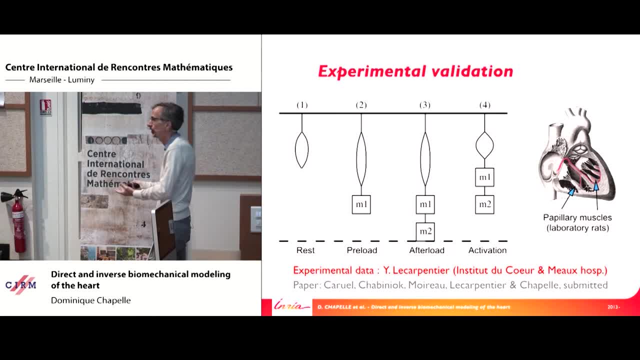 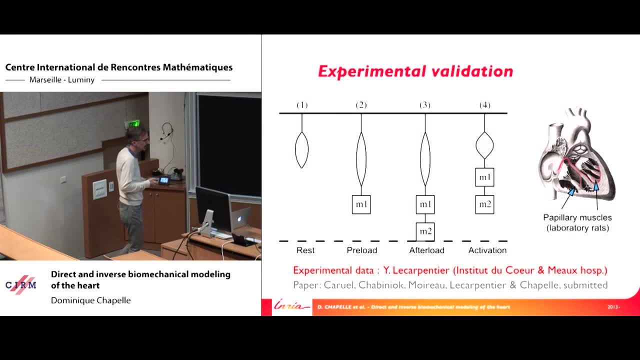 You want to check that the material, actually the active material, behaves as modeled in the equations. And then we talk about the heart scale. That is the heart scale, That is the global stage. But here for the experimental validation at the local scale, we used some data in collaboration. 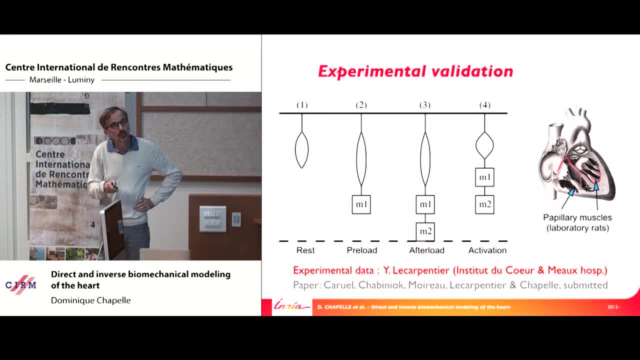 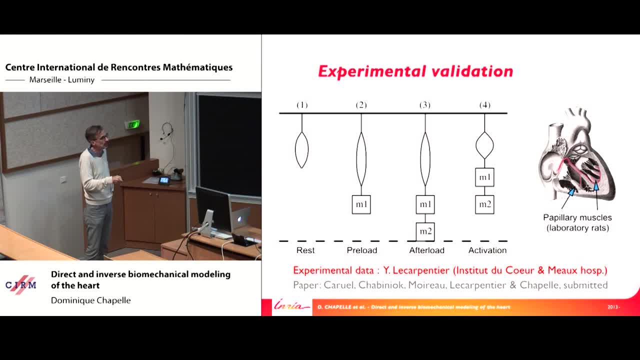 They are made of the same myocardium material as the walls of the heart, But they're much easier to deal with when isolated from the heart. They're still active when you sever them And then you submit these samples to a cycle of loading that's designed to mimic the cardiac. 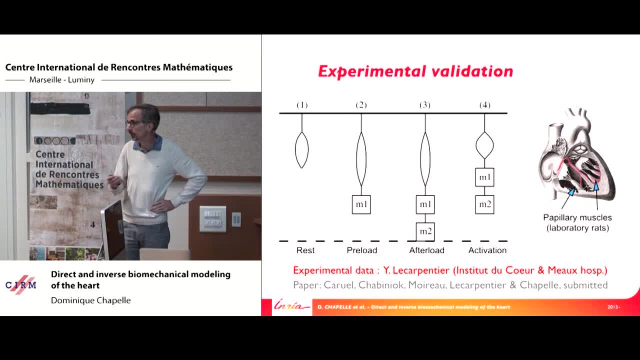 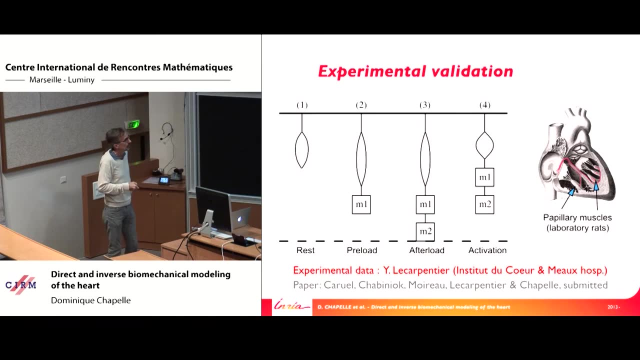 cycle. So first you extend them passively, so you have to load on them, And then you will make them contract by electrical activation And you prevent the fiber from shortening until they're able to reach a higher force, And then they shorten and they come back. 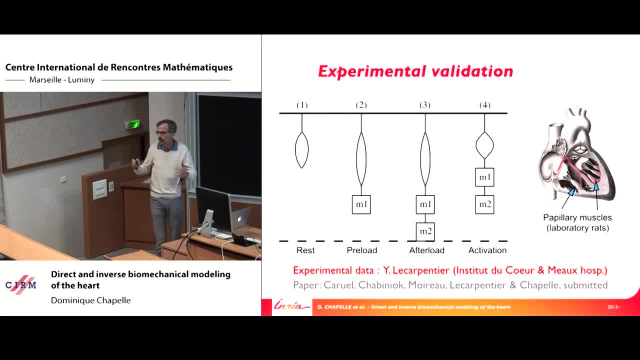 So here this would represent the passive feeling of the heart, the first stage of the cardiac cycle, And then this would represent here the Well. actually this one would represent the ejection- Ejection phase of the heart against a higher pressure, that is, the pressure prevailing. 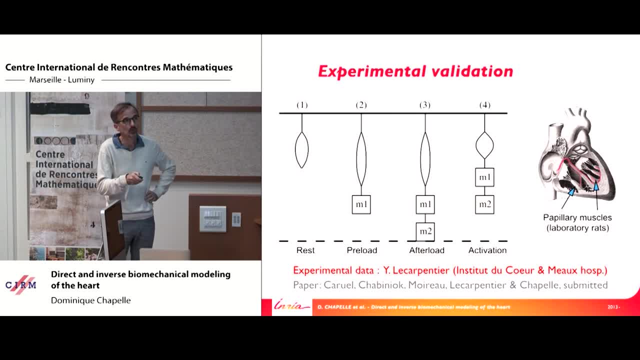 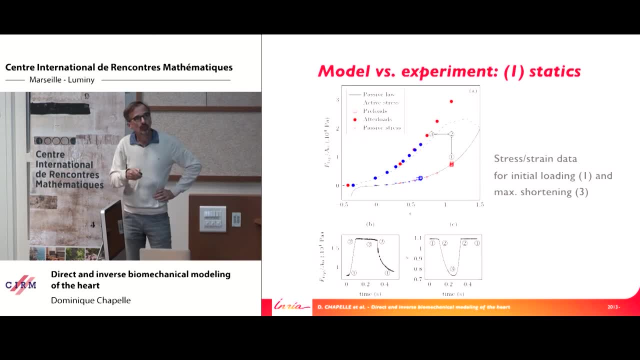 in the arterial system. So this would be the pressure prevailing in the venous system and that in the arterial system. What you measure- I forget about this figure here, but what you measure in these experiments are recordings over time of the force measured at the tip of the sample. 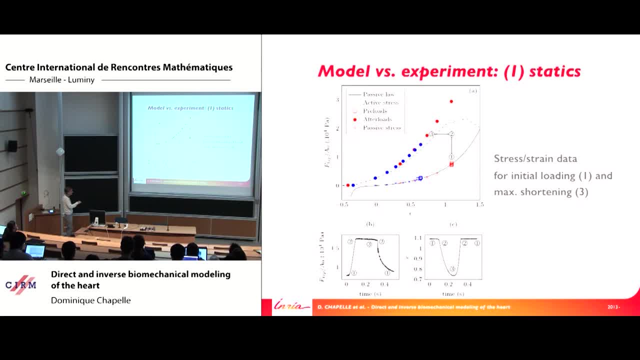 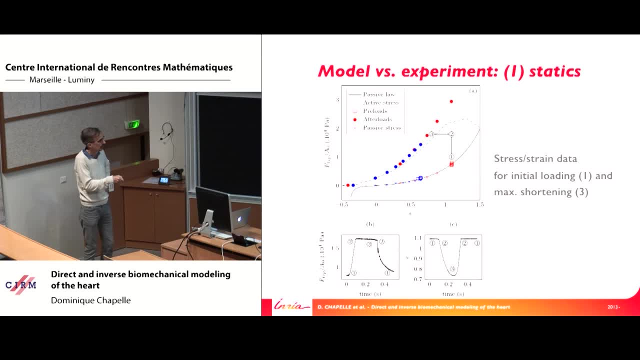 So it's limited by this M1 plus M2.. So it's limited by this M1 plus M2.. So it's limited by this M2 value that you have seen. And then shortening of the sample over the cycle, And this is what we aim at reproducing with the model which you see here. 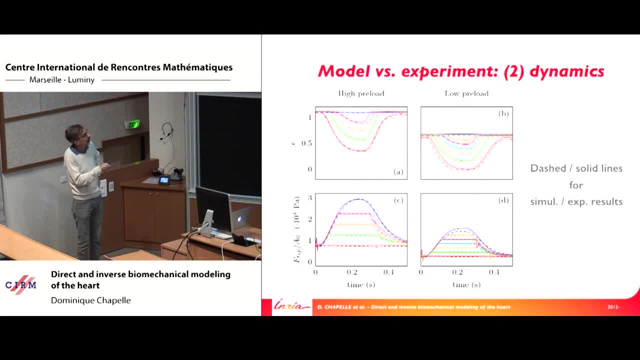 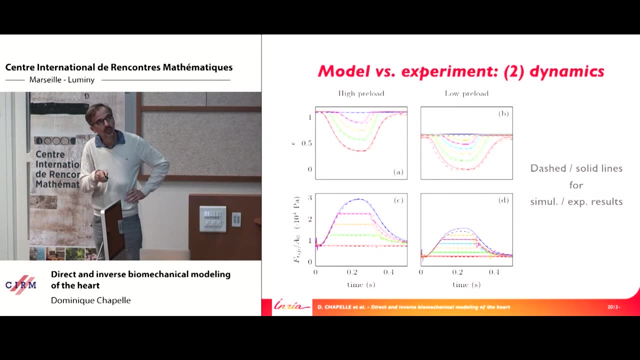 So this is a comparison over time of force and extension, so shortening in this case, against two initial loads, two levels of preload, so the M1. And then several levels of M1 plus M2. And it's a comparison, again over time, of these two quantities between simulated in. 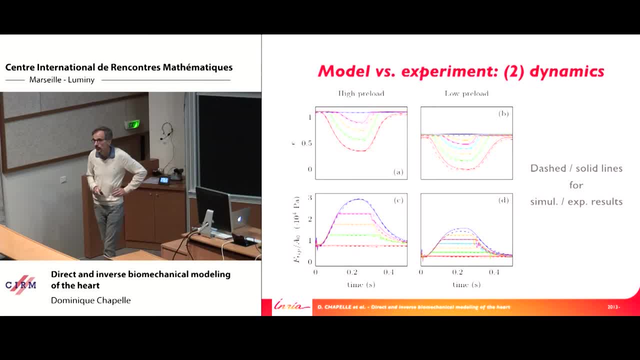 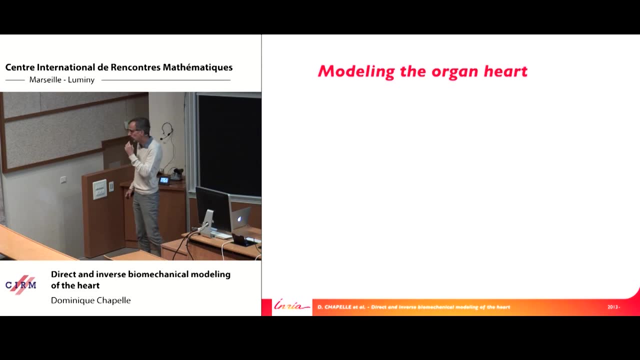 dashed and experimental in solid lines. So, as you can see, over the various types of loading, it's pretty reasonable, reasonably accurate. Now again, if you want to go to the organ scale, it presents some additional challenges, Okay, Okay. 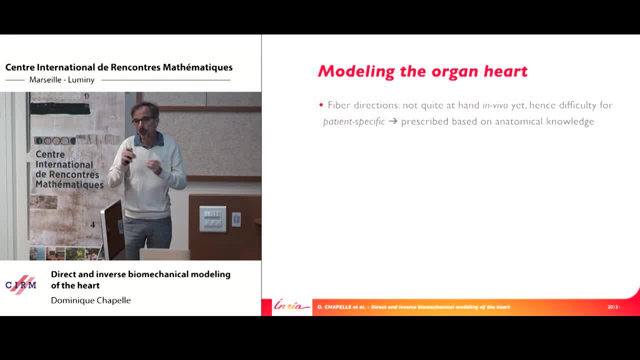 Okay, Thank you. So what we do is, in particular, in the muscle sample case, the fiber direction was quite straightforward, but in general for the heart the structure is complicated and the fiber directions are not something that you can measure in vivo. so in a patient, 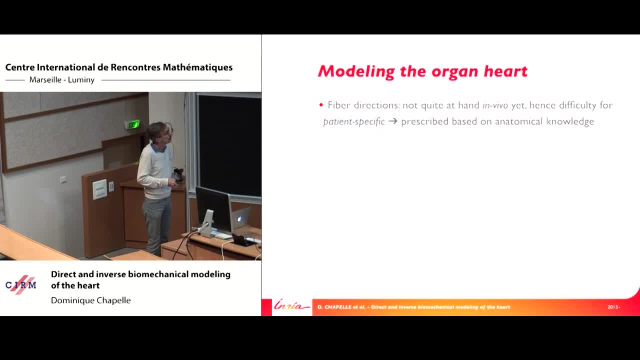 It's not something that you could actually measure. So what we do is so far because, well, hopefully in the future there will be some imaging modalities that will be able to give you fiber directions on a patient-specific basis. 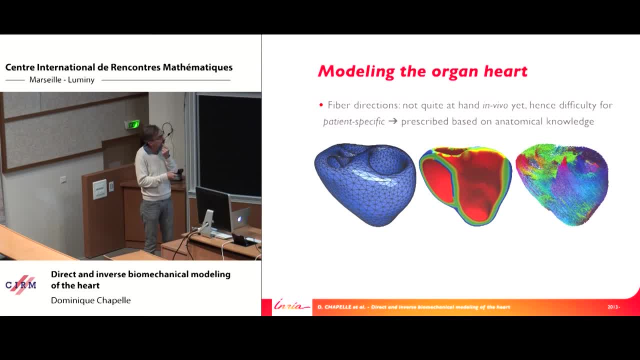 But so far what we do is prescribe the fiber direction based on standard anatomical knowledge. So typically, based on the position across the thickness of the muscle that we compute, we have an angle of elevation of the fibers that you can see here. This is the fiber direction used in this particular patient-specific model. 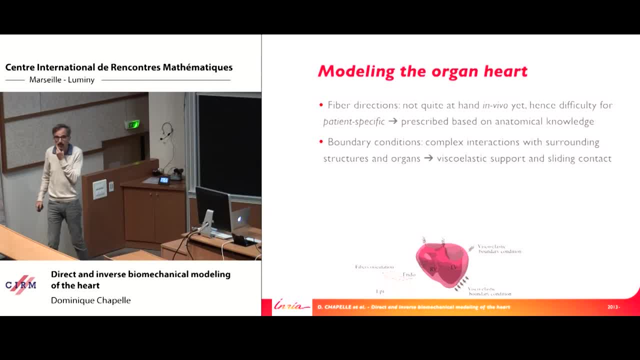 Now, boundary conditions are also something quite complex for this type of model, because there are complex interactions with the surrounding structures, for which we use a combination of viscoelastic support and sliding contact. So it's very demanding in terms of modeling and CPU time. 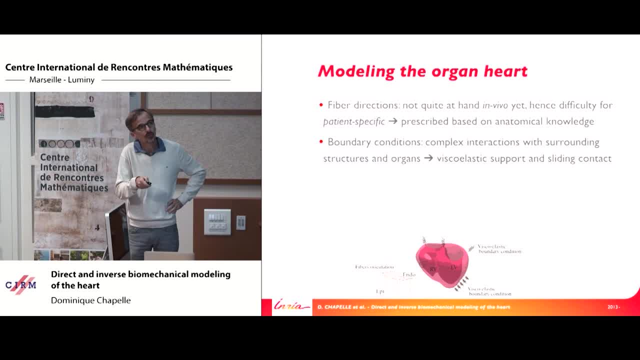 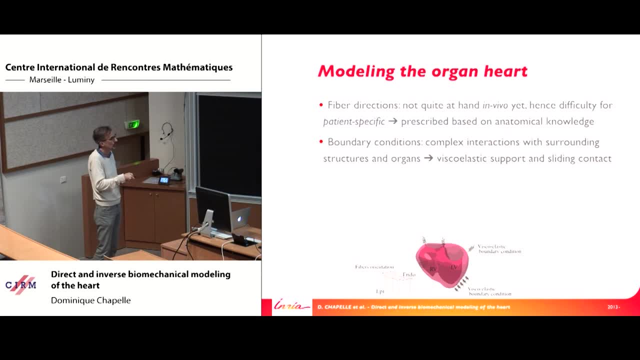 And also we have the truncation of the model, because you have to truncate your system somewhere. So here you need to substitute some artificial boundary conditions for the actual structures that you have taken out of the system, And then you also need to close the system in terms of 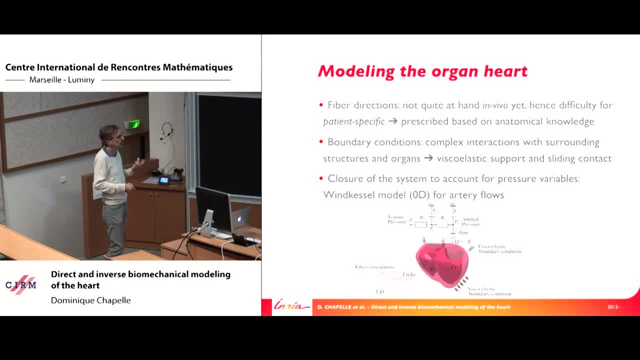 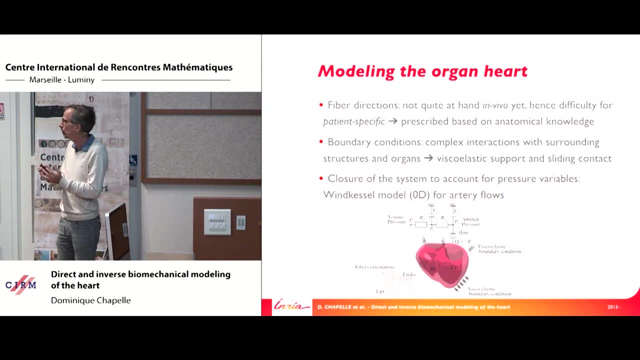 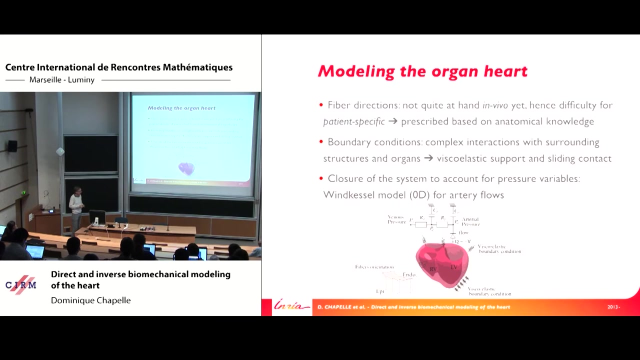 of hemodynamics, so blood fluid mechanics, Which for many cases we represent in a very simplified manner in each cavity of the heart as a single pressure volume system. So this means that you can, from the point of view of the tissue, for many applications you can consider that the pressure inside the cavity is homogeneous. 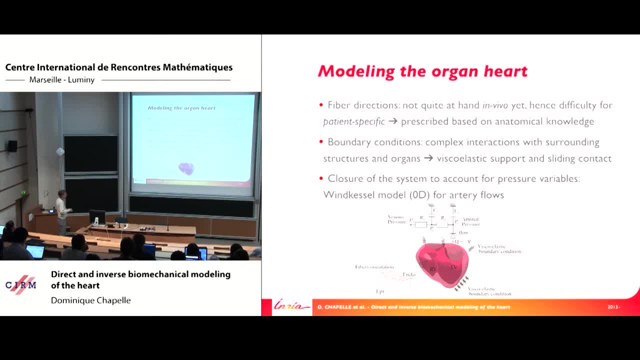 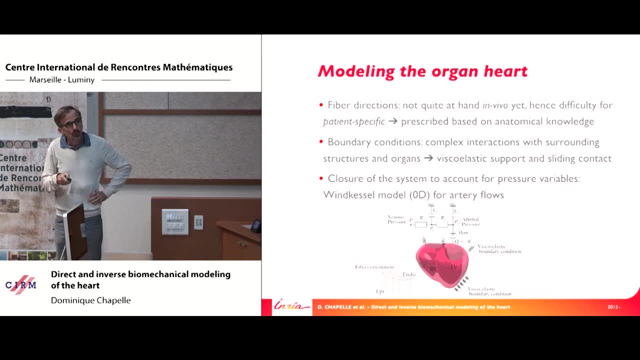 And then it's simplified. you don't need to actually consider the flow equations. For other types of applications we actually can consider these equations, But then if you take the cavities as single pressure volume systems, then you can also close the system by using simplified modeling of the outlet. 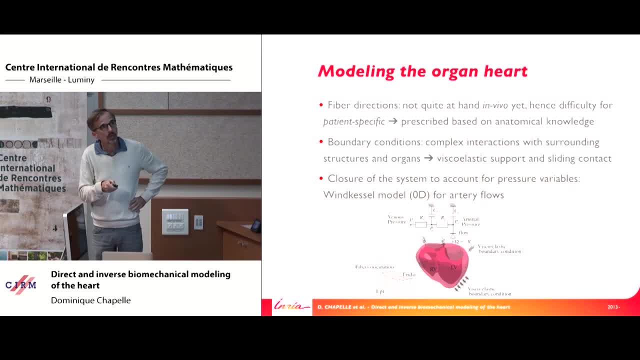 So the arterial network, by equations. These are the equations that are obtained as analogies to electrical circuits, So the combinations of resistances and capacitances outside of the heart. So this would close the system in terms of outgoing flow and pressure sitting at the outlet of the heart. 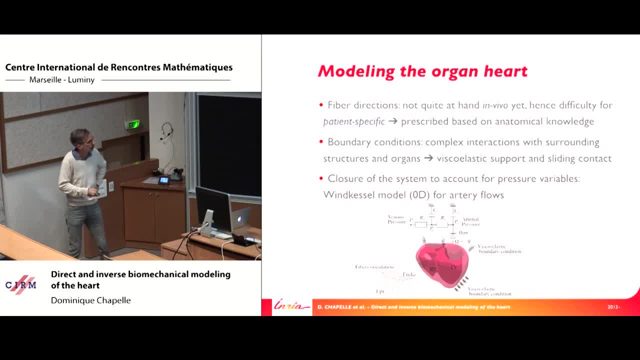 These are called Winkessel models in this type of application. So a set of 0D that is ODE's. And now we also have some difficulties with the reference configuration, Because in practice you never see the reference configuration in an actual heart. 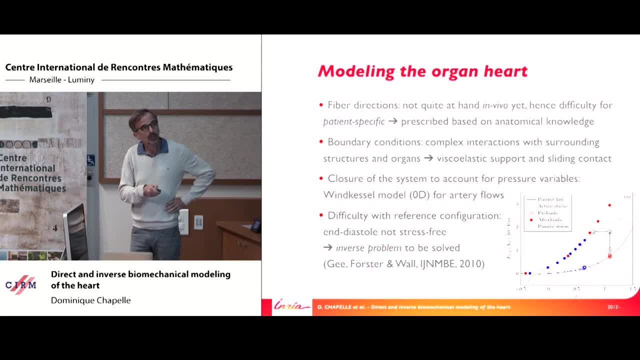 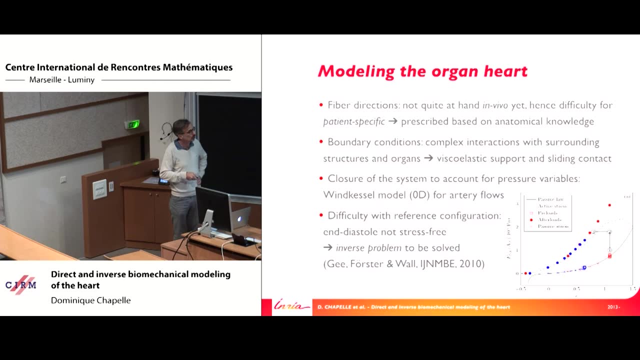 It's always moving, say, In particular, the one that's the most still at the end of filling is, of course, not stress-free Because it's inflated due to venous pressure. So if you want to find the reference configuration, that is again the stress-free configuration. 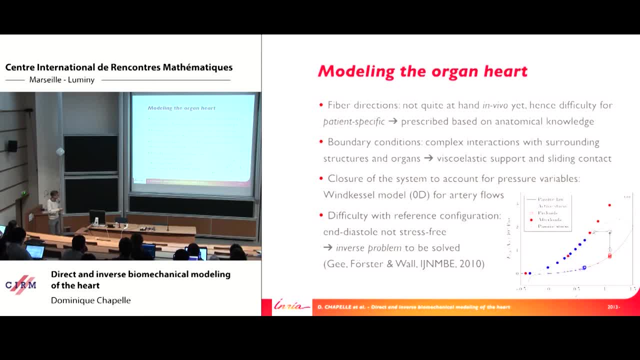 you need to solve the inverse problem, to find the configuration in which stress is vanished, And this is difficult. well, not only because it's an inverse problem, but also because it's ill-posed, in this case, due to what you see here, this curve. 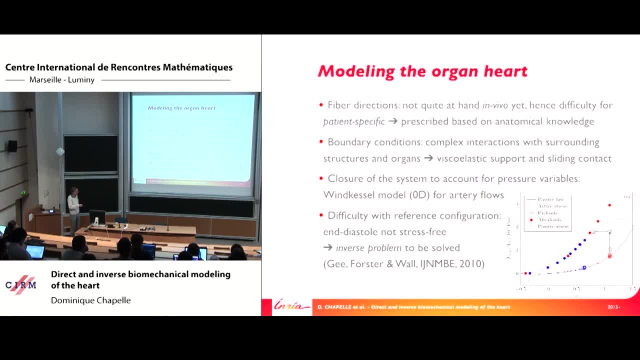 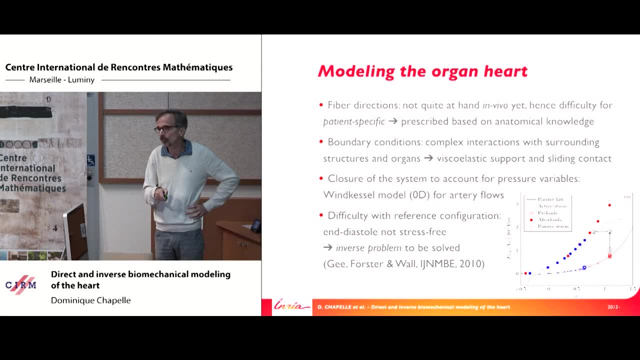 is the curve that represents the passive behavior of the heart. So force against extension, This is zero stress, And you see that it's extremely soft near the reference configuration. So of course it means that it's very difficult to get here by an inverse problem. 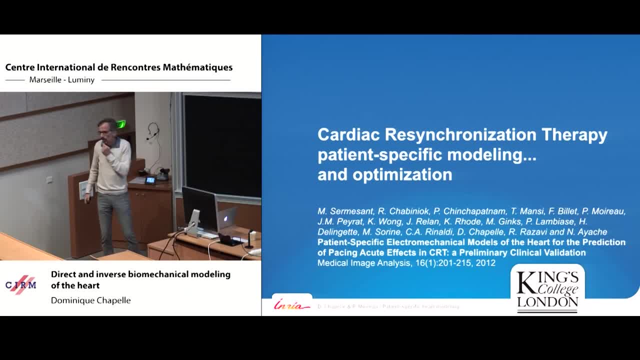 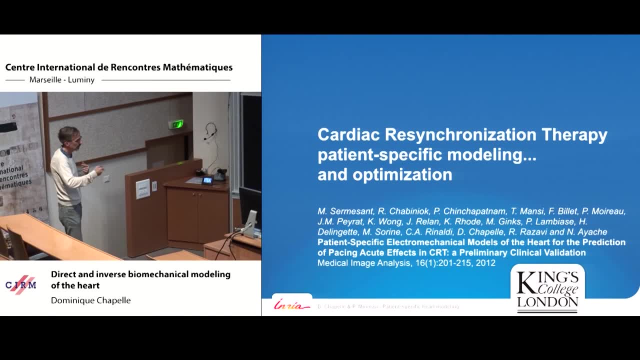 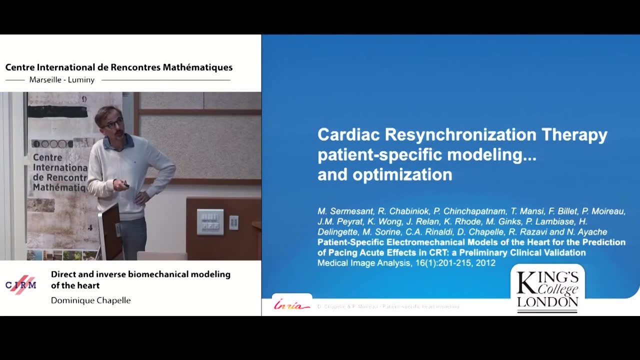 It's very ill-posed. Okay, now let me show you the type of validation that we can obtain at the end of this path of modeling, And this is: These are some trials that we made regarding what I mentioned before as cardiac resingulation therapy, in collaboration with 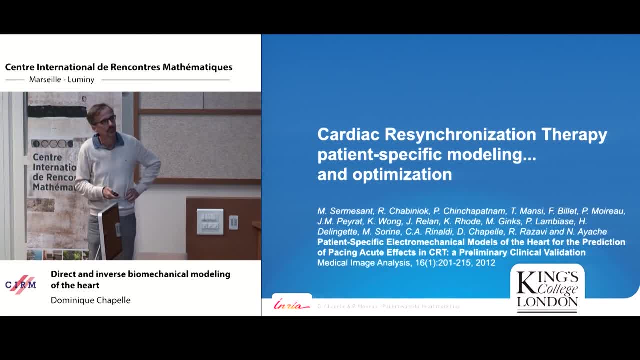 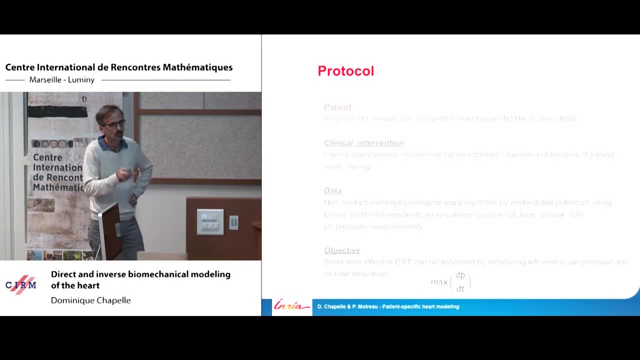 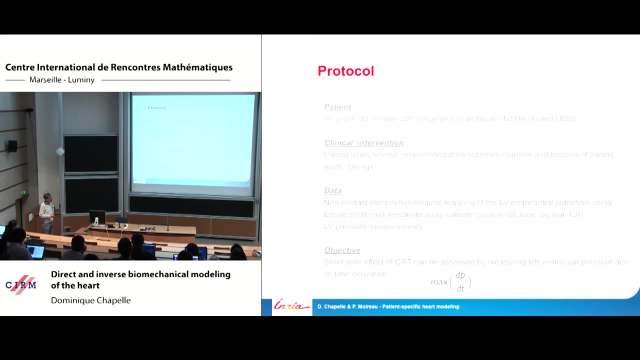 in collaboration with clinicians from King's College London. Okay, this is the detailed protocol, but let me explain it in a few words. What happens is that for certain types of patients, the activation of the contraction is quite heavily desynchronized due to some pathologies. 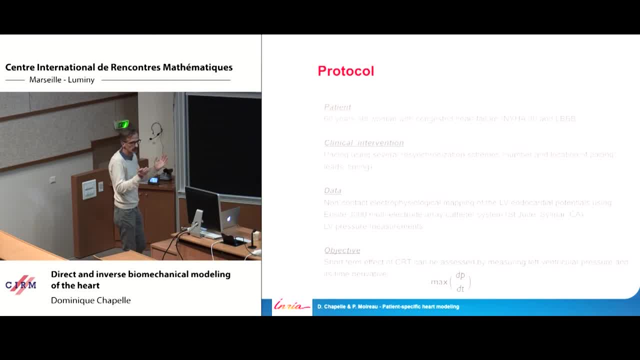 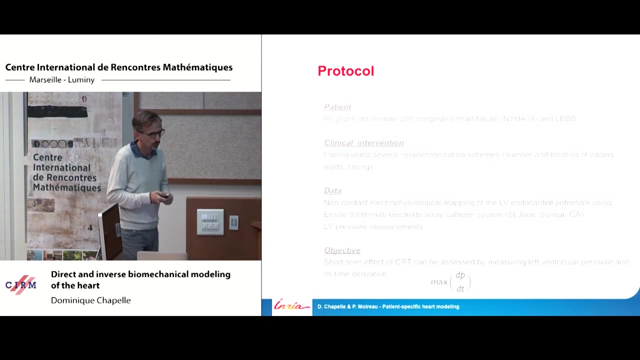 And then, of course, as you can imagine, the contraction is much less effective than with a healthy heart because it's desynchronized in the way that active stresses are built. So these patients suffer from severe symptoms- heart failure typically- And the way you can try and cure them. 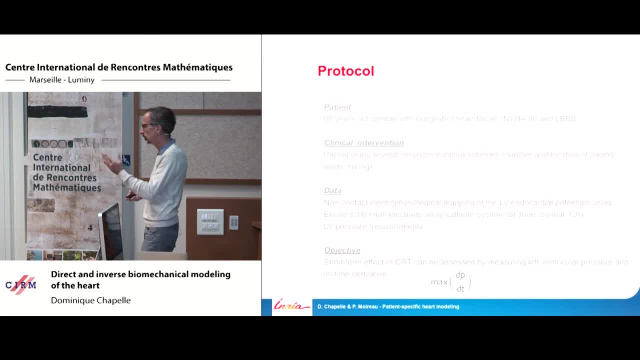 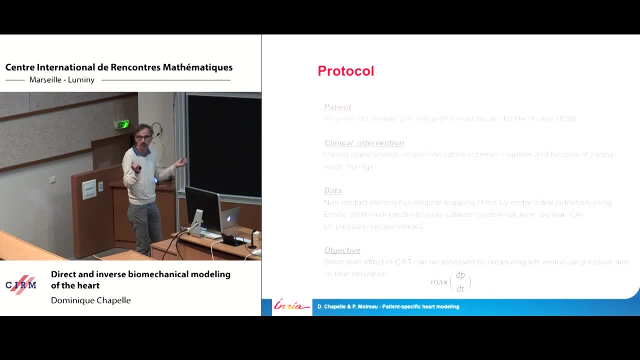 is by using this type of therapy- CRT, cardiac resynchronization- to resynchronize the contraction, And the way you do this is use a pacemaker with several electrodes to activate the heart. The contraction is in a more synchronized manner. The problem is that it is estimated that, at least for 50%, 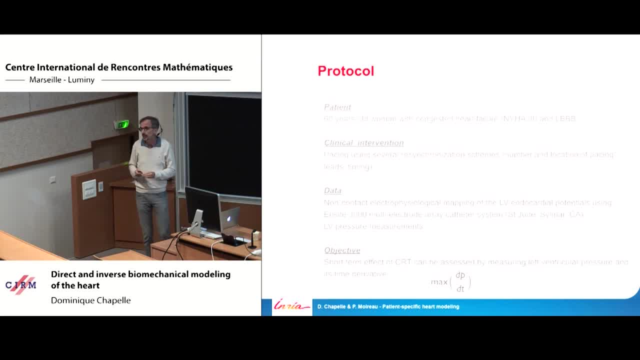 if not two-thirds of these patients. there is actually no response, no benefit from the therapy. So it's a heavy and expensive and risky therapy To actually go and place these electrodes on the heart or in the heart in some cases And for at least 50% of these patients. 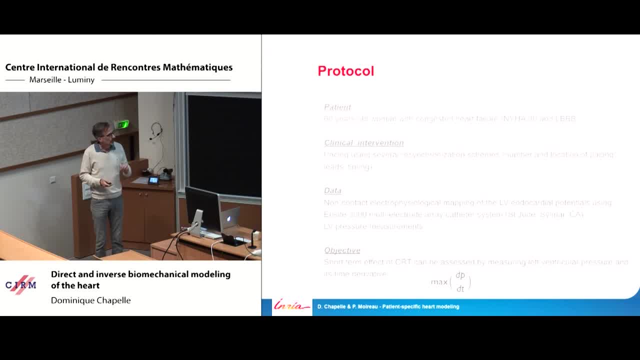 there is no response, no benefit. So here what's at stake is the possibility, the perspective of using modeling- patient-specific modeling, so models of a given patient- to at least detect people who will not respond to therapy And of course also hopefully optimize the therapy. 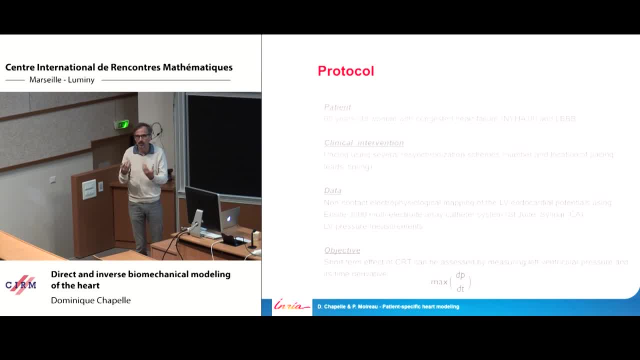 for each specific patient. So decrease the rate of non-responders by using the model to tailor the therapy At this stage. of course, this is preliminary, what we have done, So it's a validation stage. So what we looked at, 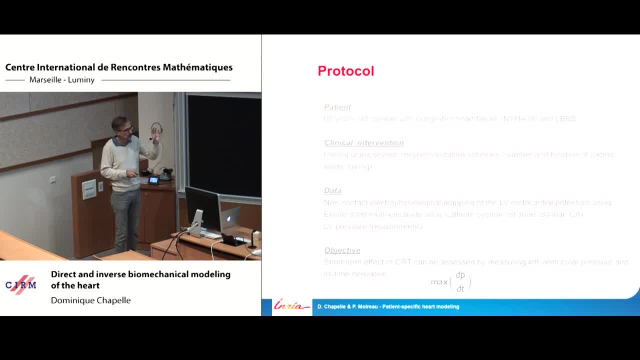 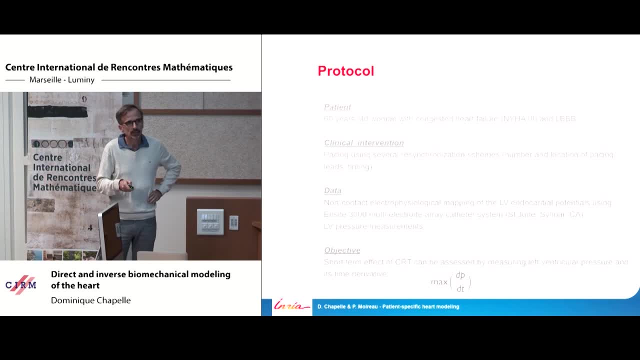 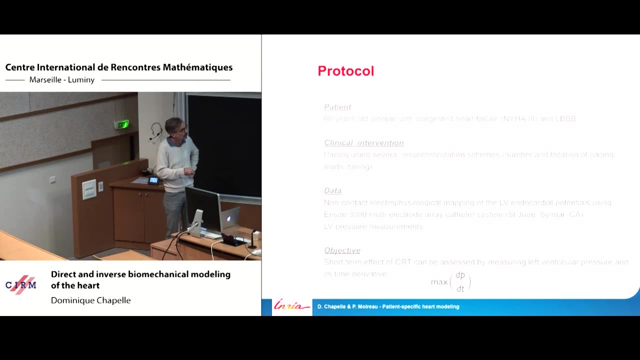 was how the model could be used to reproduce what was actually measured in a patient. So this is what we focused on, And the main indicator that's used to assess the success of the therapy is by looking at the pressure inside the left ventricle. 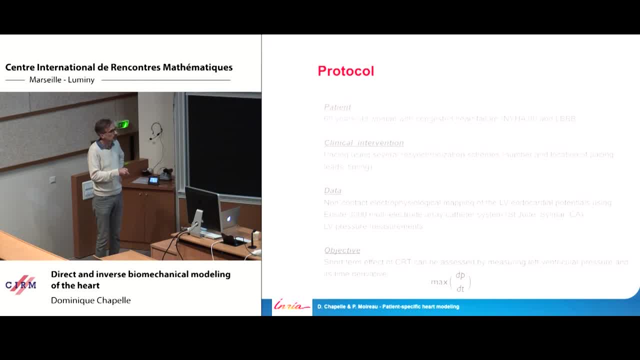 so the main ventricle, The increase rate of this pressure. you take the maximum, So maximum pressure increase rate And of course, the more effective contraction is, the higher this indicator should be, And this is what cardiologists use. 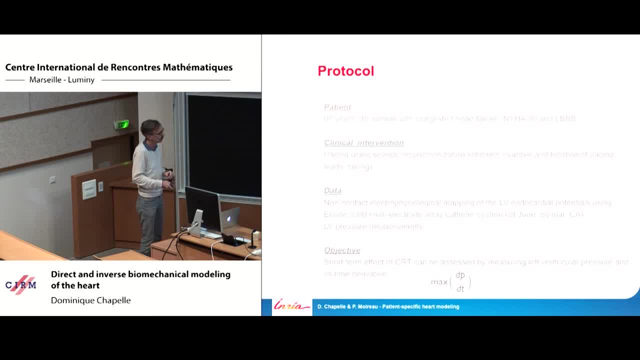 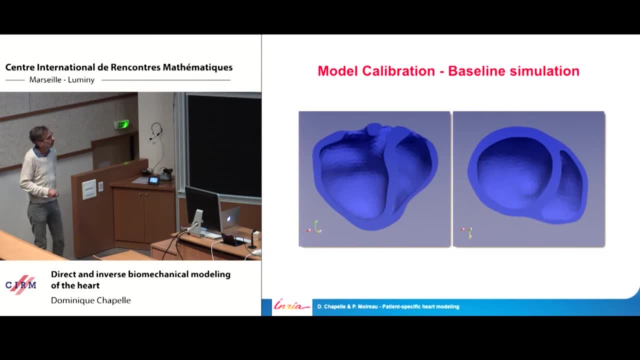 and this is what we will use as an indicator Now for one patient. this is the patient-specific model that was constructed. So here you have two cross-sections of the heart, so-called long axis and short axis. left ventricle right ventricle left right. 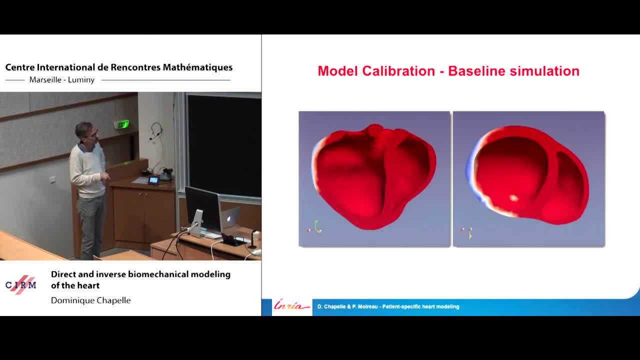 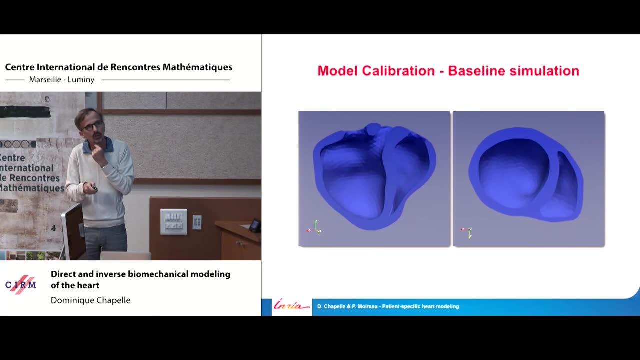 And what you can see. so the electrical activation is: the heart is in color and you can see that visibly. so of course it's in slow motion, but even so it's very visible that the activation starts in the right ventricle. 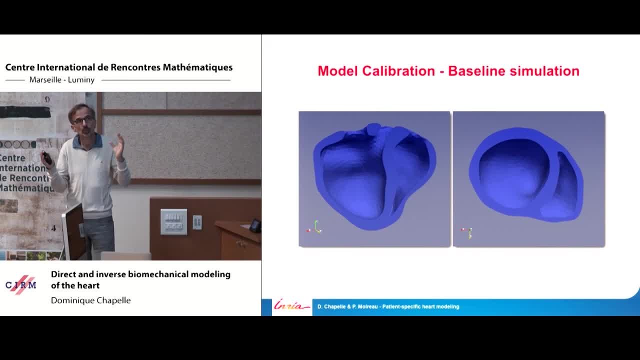 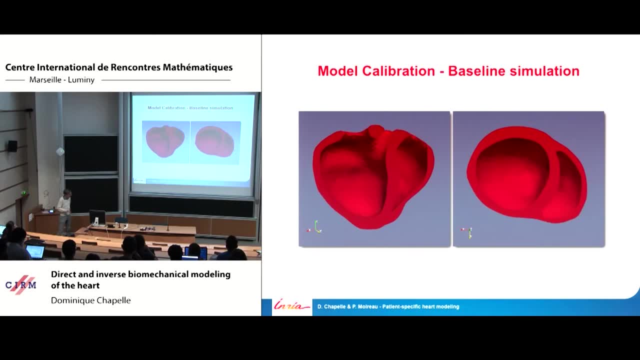 and then propagates to the left ventricle. This should be much more synchronized in order to have a healthy heart. So it's a typical indication of CRT: this patient, This is the model, So complete heart cycles all the way at the end of the modeling path. 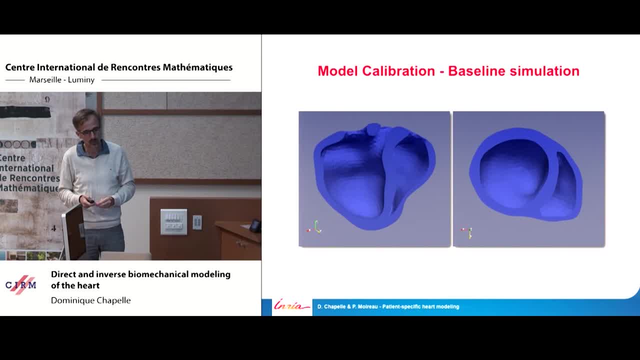 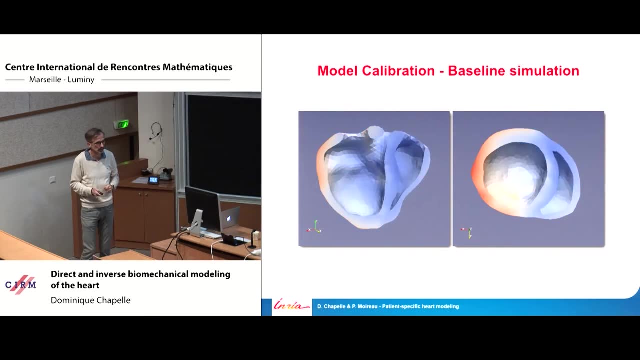 that I summarized in the first part of my talk. So this is the patient before therapy. How can this be validated? Well, we have lots of measurements. We have the pressures inside the ventricles. We also have medical imaging. so this is the first time that you will see. 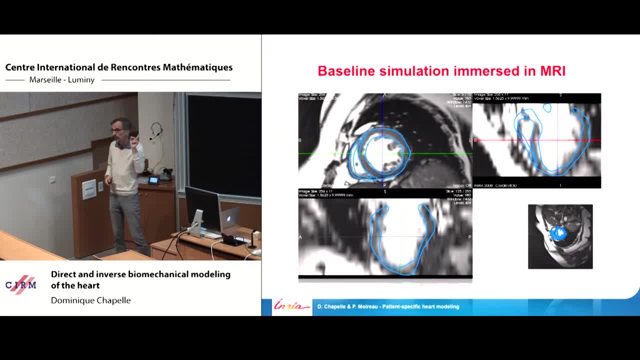 you'll see more. This is an MR sequence, in this case in three sections, and it's compared to the boundaries of the model in blue. So you can see that in these two cross sections- the main ones again- the model follows quite accurately. 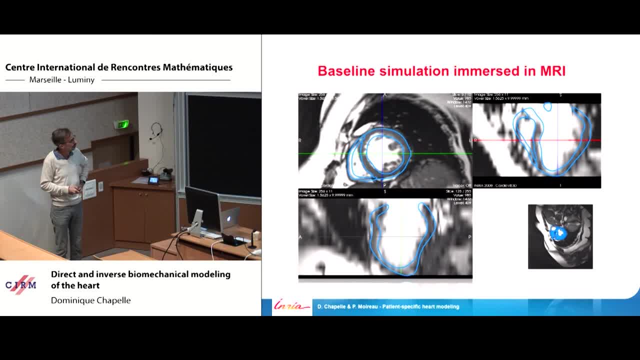 what's measured in the imaging. Of course, as you could say, this is the result of calibration. So we tweaked. We tweaked all the parameter, models, boundary conditions, everything that I mentioned, to obtain this good adequation, including for the pressure. 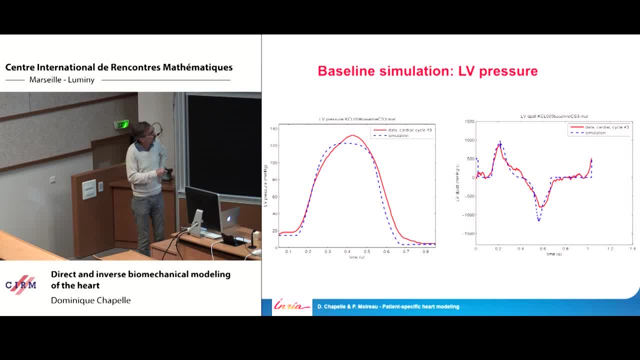 So this is the pressure inside the left ventricle. It's not perfect, but the peak of DPDT that's here is close to data. It's simulation in dashed blue and data in red solid. So this is the part that we will look at. 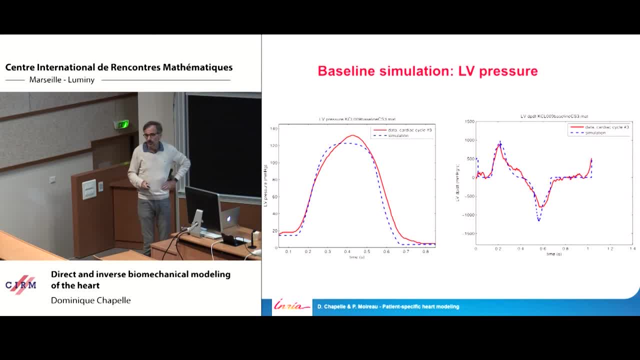 this peak of DPDT. So again, everything was calibrated. but now what's extremely important is that we will not change the calibration before we apply the therapy in silico. So we will try and prescribe the same electrical activation as corresponds to the therapy. 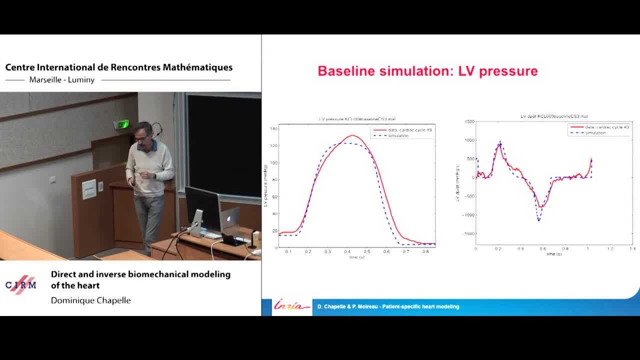 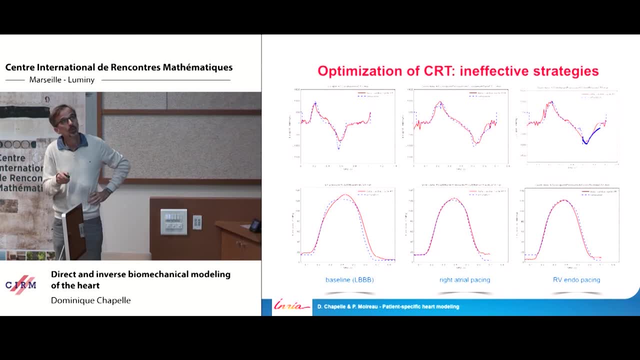 in the various strategies that were actually tried on this patient. First cases: here are the therapies that proved to be ineffective for this patient. So this is a patient before therapy baseline. We had this level And for these two therapies the DPDT max was not increased. 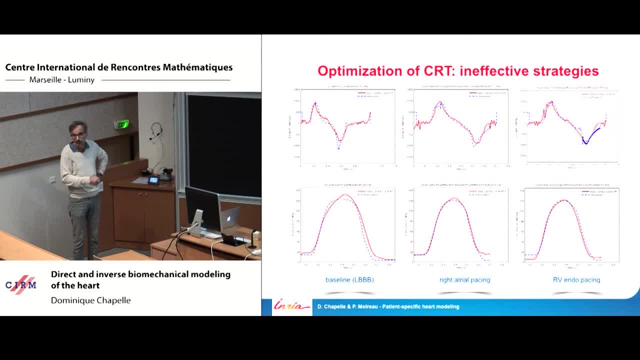 And again, the model shows what is accurate, is close to what was measured. This is extremely important because here it means that the model is able to detect non-responding behavior. So it's very clear to the therapy. And now these two. 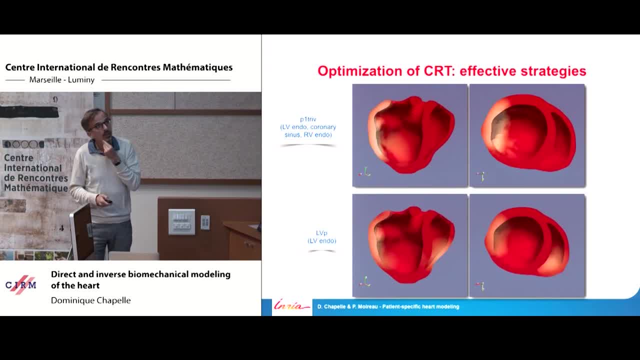 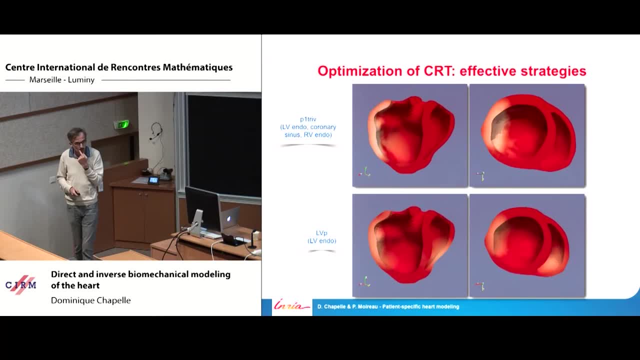 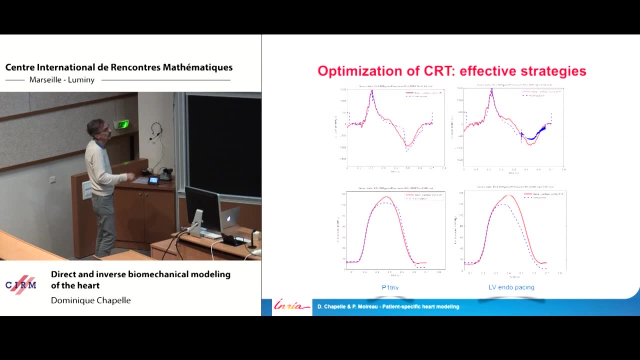 resynchronization schemes here would be strategies that were actually effective for this patient. So here you see the corresponding models with the activation, again in colors, And here the DPDT max that was obtained for these two cases. Again, it's the same patient with several strategies. 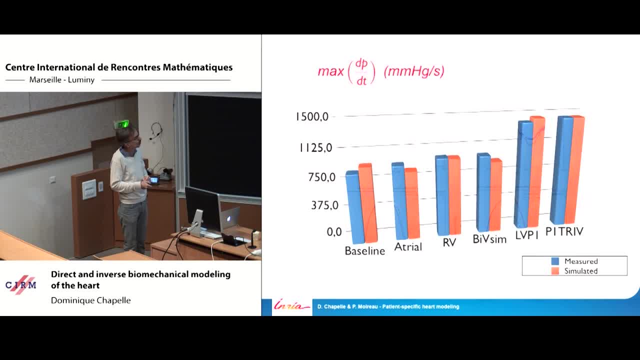 that were tried, And this is a summary of DPDT max, measured versus simulated, for this patient: Okay. so this is very nice in this case, But it's a single patient, So of course, it requires much more validation. That is actually taking place right now. 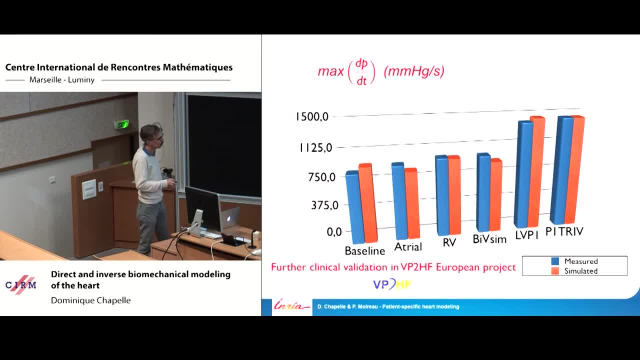 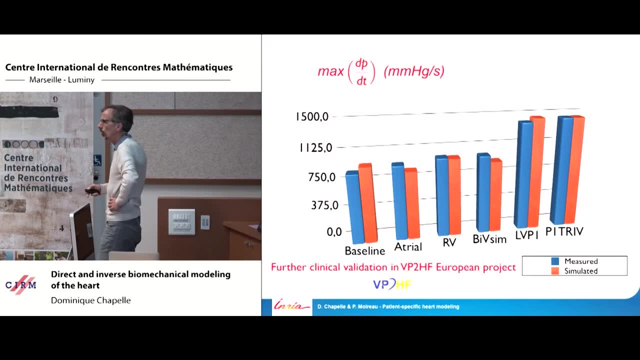 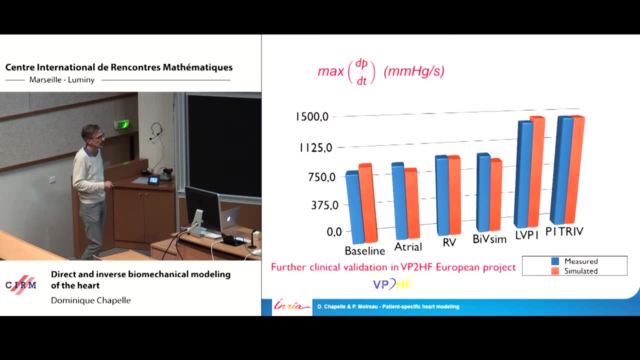 within a European project that's called VP2HF, in which we take part. So in this project, approximately 100 such cases were actually considered, with the data collected specifically for the project, And the same type of validation is actually happening right now. Okay, so this is for. 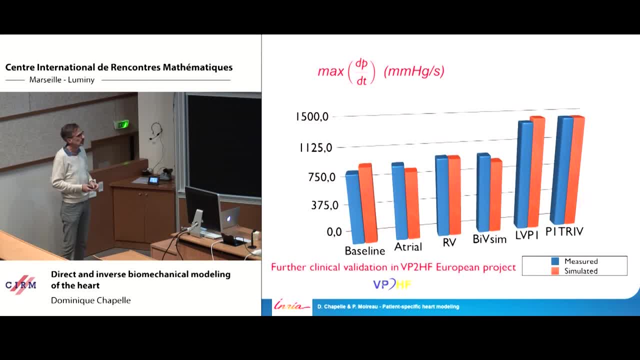 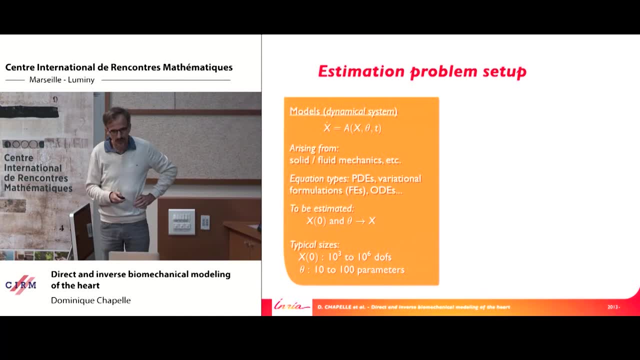 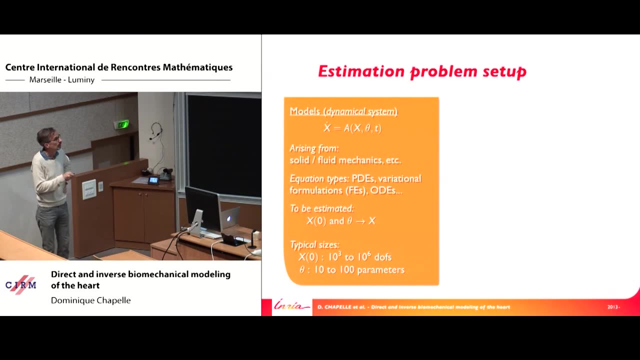 the direct modeling all the way to clinical application. Now, as I mentioned in the beginning, I want to talk about something else. in the remaining 15 minutes or so I want to cover inverse problems pertaining to patient-specific type of motivations, That is, the estimation problems. 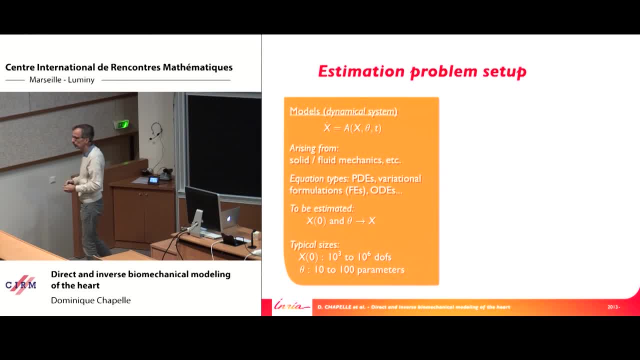 that you need to solve in order to adapt the model to a patient. So the types of models that we have, as you have seen, are dynamical systems that we can summarize in a very compact form like here. So dynamical system X would be the state variable. 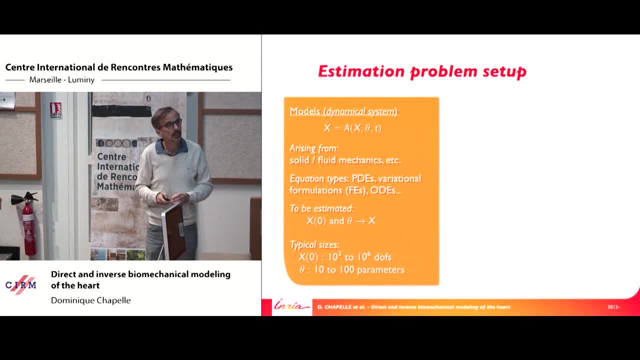 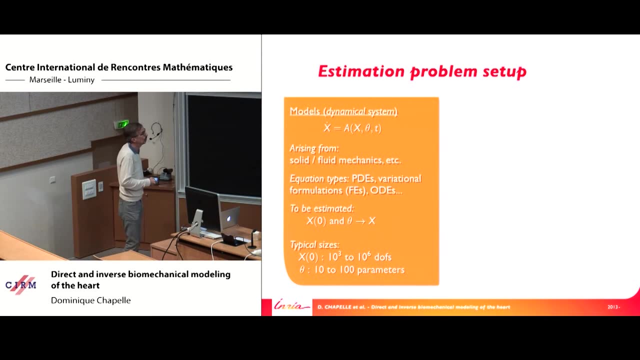 So typically the displacements at each of the points in a system. Theta would be a set of parameters that are unknown or uncertain so that you need to adjust in order to have a proper dynamical behavior. The equations that would be summarized here are typically of PDE type. 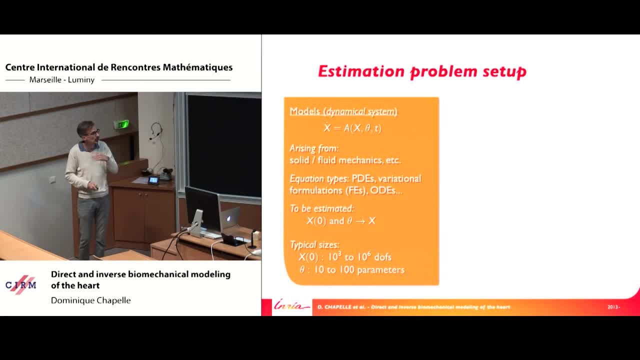 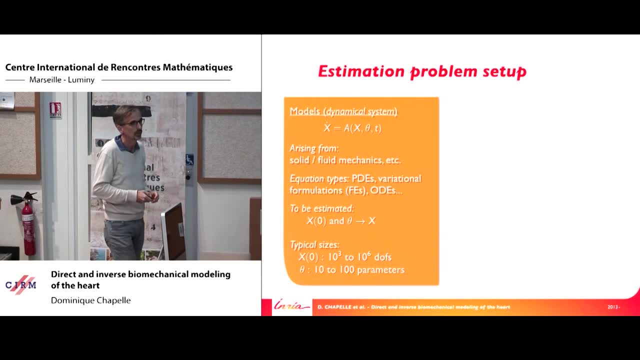 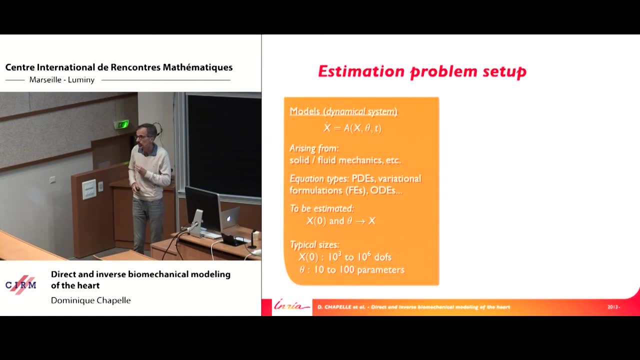 So they would, in particular come from the rational formulation that I showed you before Sets of ODEs, for example for the simplified fluid models that I mentioned in my modeling part. So it's a combination of equations that you have here. 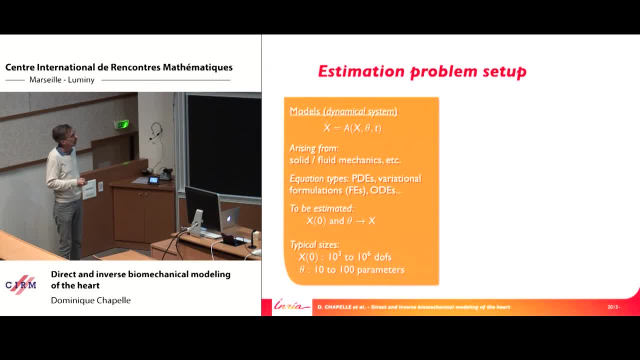 But again, it's heavily PDE based And what you need to estimate in order to simulate a system that will be close to the actual system is the initial condition. always, In a dynamical natural system like this, you never know what the initial condition is. 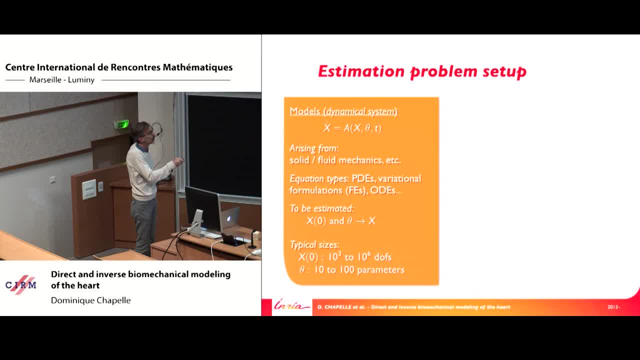 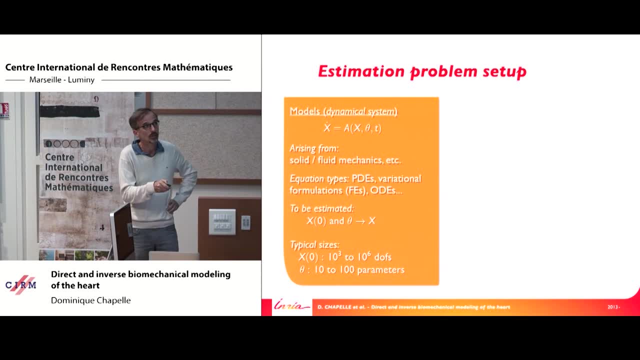 And you need to also know, adjust a set of parameters- Again the theta vector- in order to obtain the trajectory. Now, the assumption that we have, and it's quite valid in practice, is that we have a much higher dimension in a state. 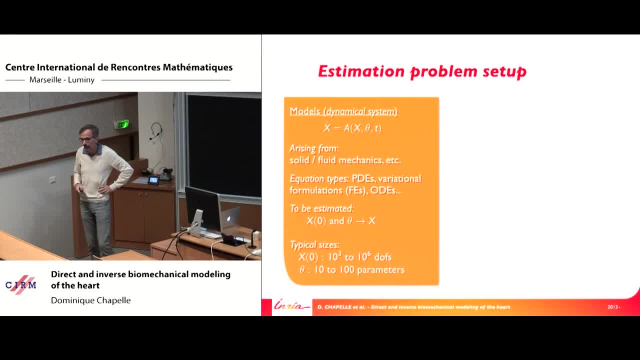 So typically, what you need to estimate here would be from a few thousand to a few million degrees of freedom, Whereas in theta, well, essentially, it's kind of reasonable to estimate from, say, a few tenths to a few hundred parameters. 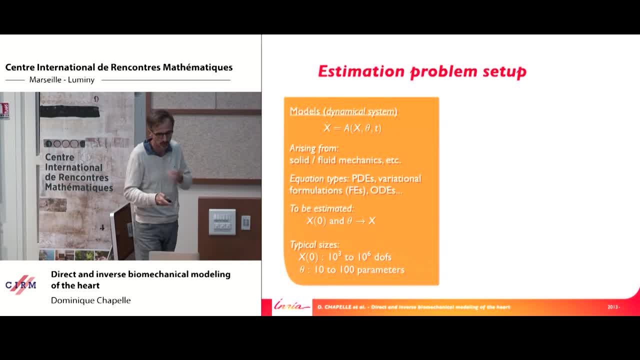 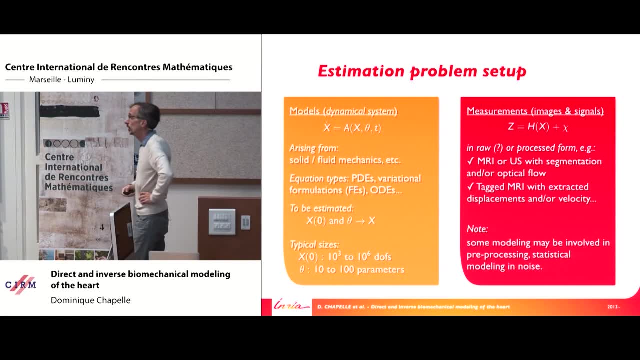 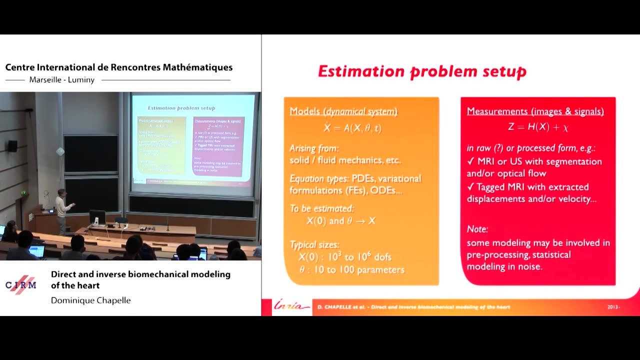 So very different dimensions in the two vectors over there. Now, to cope with this uncertainty that we mentioned, you have actual measurements on the system, Measurements coming from various images and signals that you can model based on the state variable. So Z would be the observation. 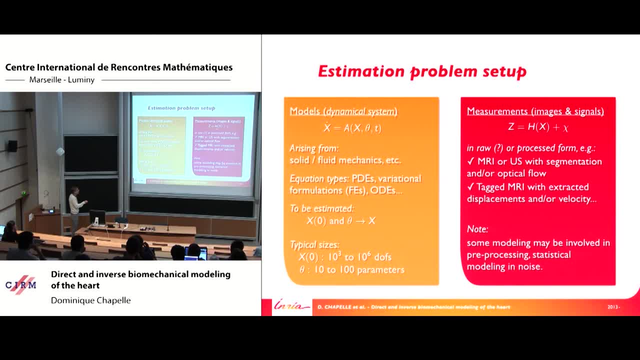 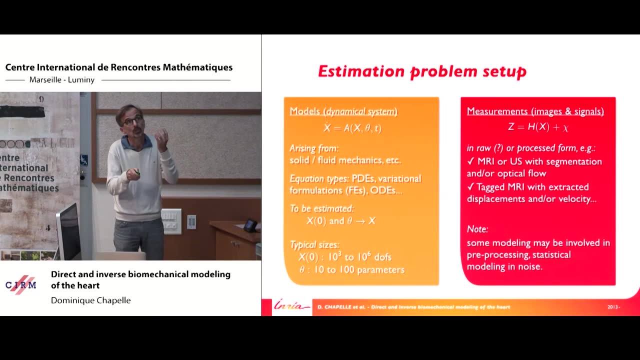 the measurement vector, And then you can formalize the measurement process by this observation operator H, And of course you have always some error in the measurement process. That's denoted by key. This operator would represent the measurements either in a raw: 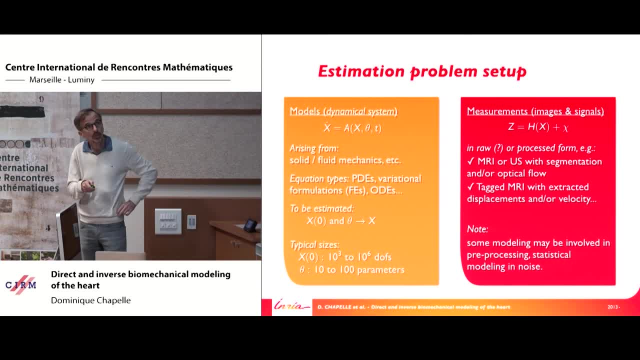 but most probably in some kind of processed form. And this would summarize Here. we had a lot of equations summarized here, And here again we have a lot of measurements summarized, in particular medical imaging. That's, as you can imagine, not straightforward to formalize like this. 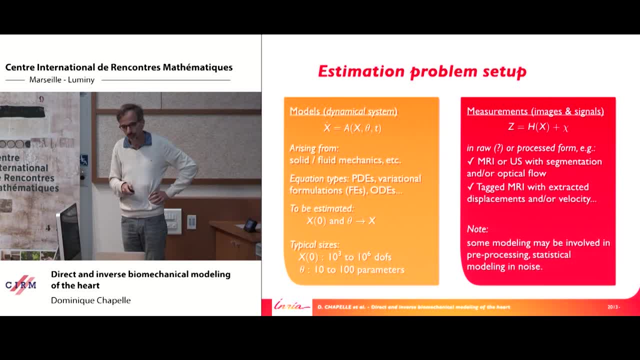 I cannot dwell on this in this talk, And it's important to recognize that this again includes some modeling. Whatever happens in the processing, this is a modeling equation that models the measurements, So in a way, we have models on the two sides. 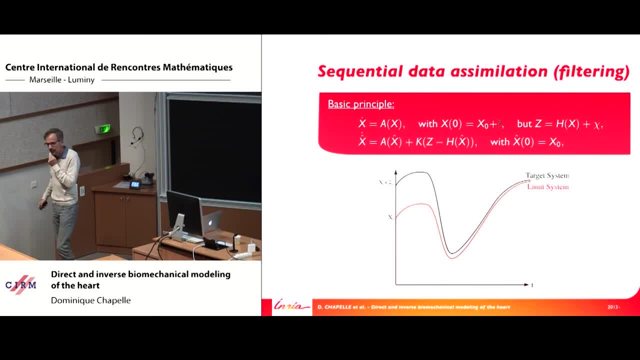 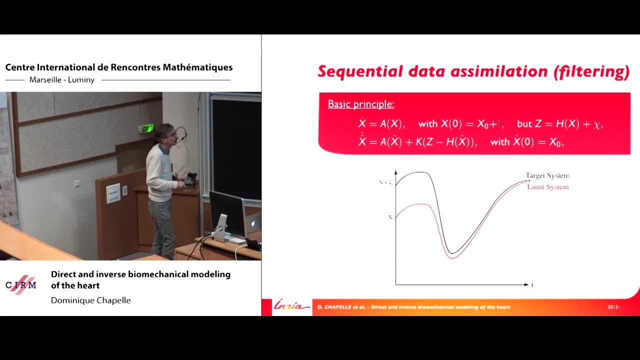 Now estimation. we look at this from a sequential data simulation point of view. This is also known as filtering. So data estimation means that we're going to use some data available in the system to reduce the uncertainty and actually track the system in time. 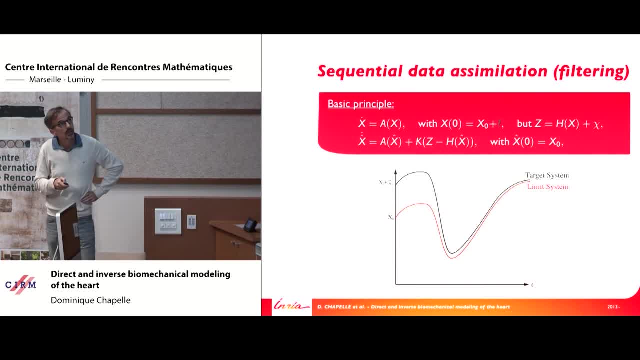 Now sequential means that, Well, this is the basic principle. So you're looking at a dynamical system in which you, at least, don't know the initial condition. So you have an uncertainty and initial condition, but you have measurements. And now 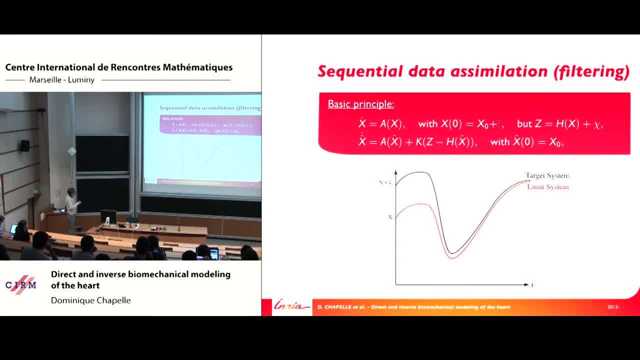 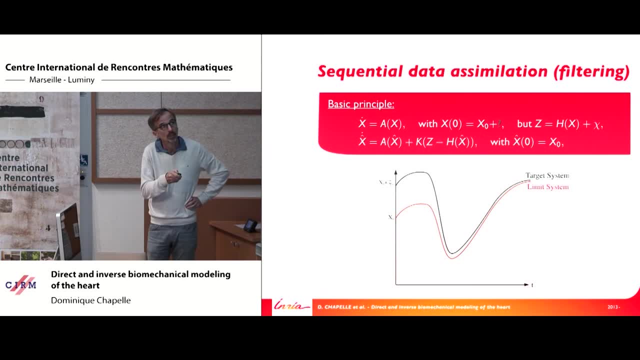 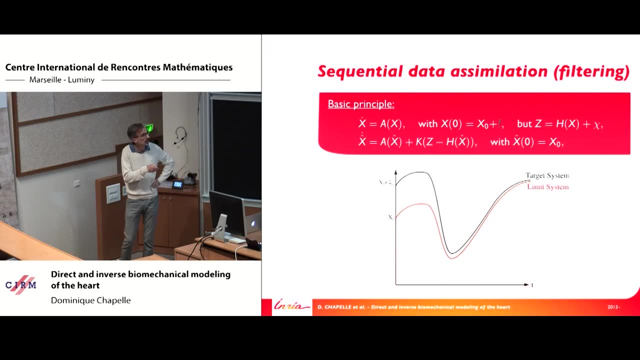 the principle of sequential data simulation is that you are going to simulate a system that mimics the actual system that you're looking at, But you correct the system equations by a term that takes into account the discrepancy between the measurements and the simulated system. So you can simulate a system. 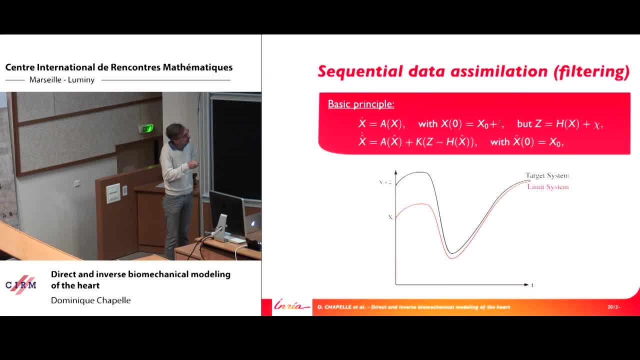 that mimics the actual system by the observation operator, And what you want is to design this gain operator K here the gain of the filter, in order to. So this would be the actual system, And the system that you simulate will start from the a priori initial condition. 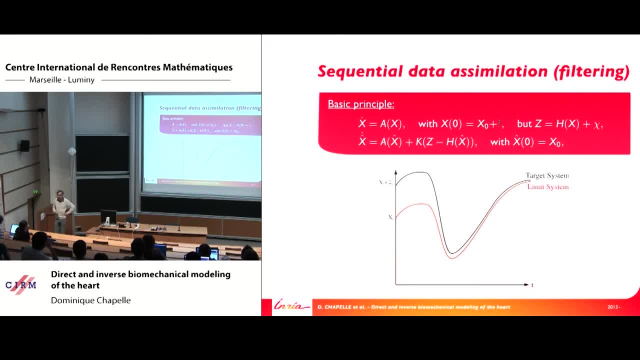 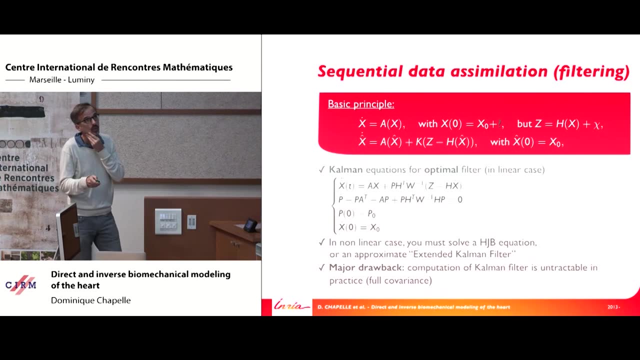 So you have an error here, But you hope that with this correction in a dynamics you can converge to the actual target system. So how can you achieve this? Well, this was formulated by Kalman for a canonical case of a linear system. 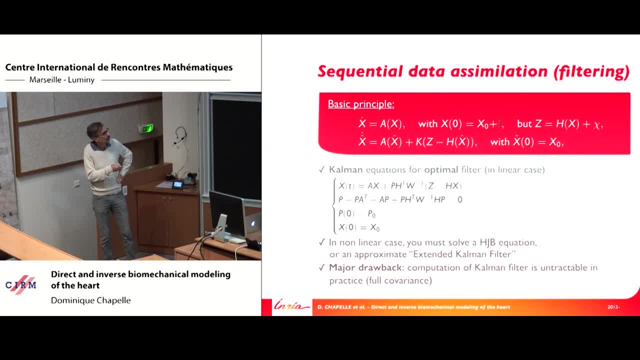 And then he formulated this type of filter in an optimal setup And this would be the continuous time Kalman equations, which can be also extended in a nonlinear system By various means. But the major drawback is that the computation of this filter that sits here 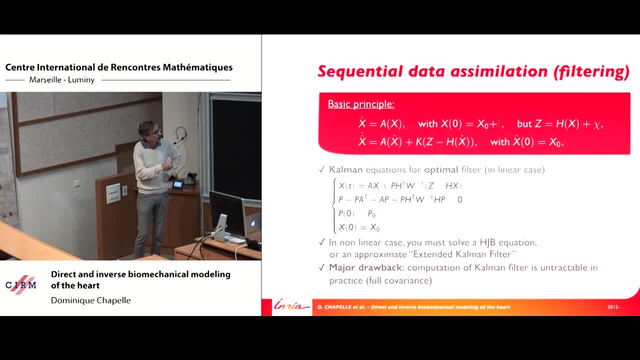 the K would be: this here uses the so-called covariance matrix P of Kalman And the covariance operator or matrix has the size of the state and is full. It has no reason to be sparse like a usual physical operator. So P in a system like a. 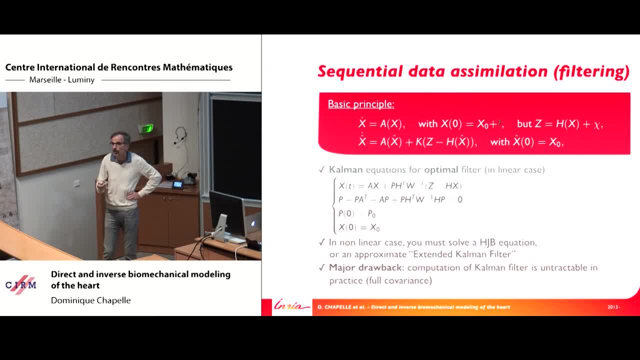 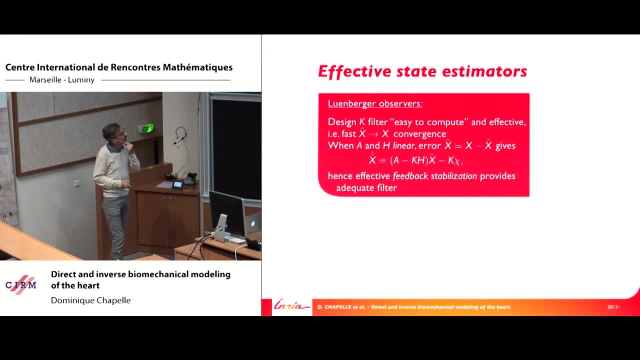 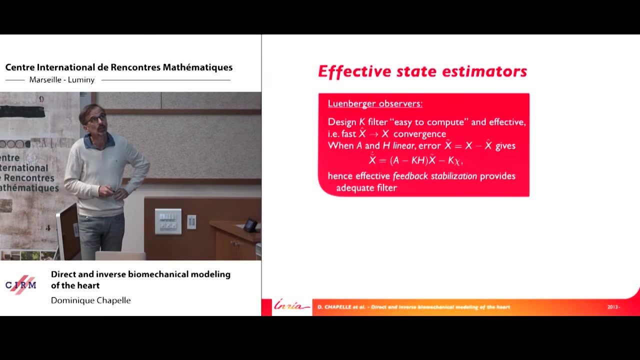 we are considering here is not something that you can compute or even store actually, given the sizes of the systems. Now, another type of an alternative to this type of optimal filtering is given by the theory of Lohenberger: Lohenberger observers. 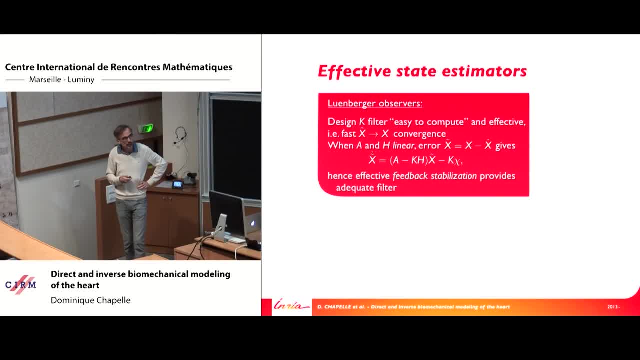 So the idea here is to design K as something much easier to compute but nevertheless effective, And what you want is to have convergence of what's called the observer X hat, so the virtual in silico system, simulated one, to the actual system. 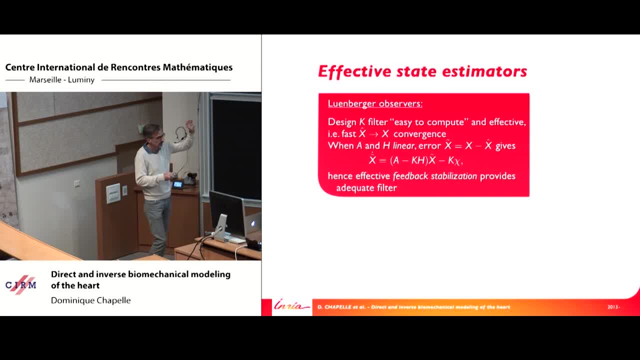 The way you can look at it. so if you take on the previous slide, you take the real system and the observer system with X hat and you subtract them, so you obtain the system satisfied by the error X tilde and you get 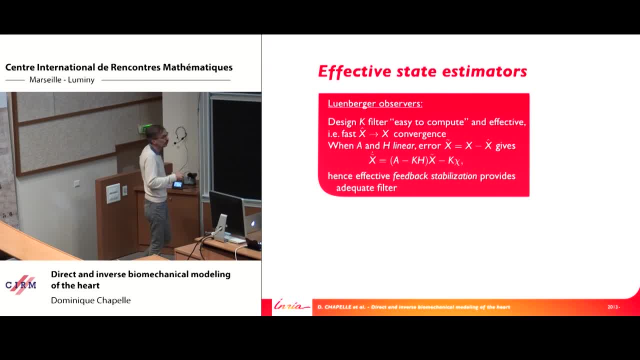 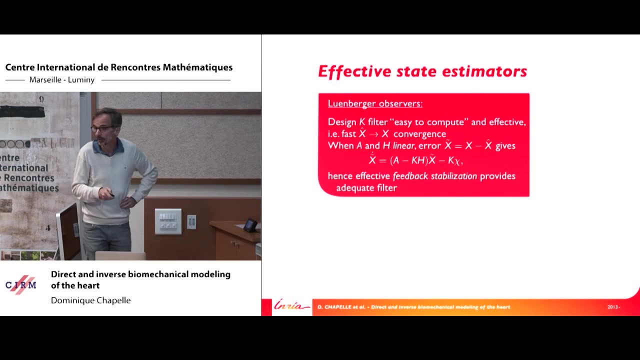 and what you obtain is this equation. And for those who have some background in automatic control, what you will recognize is the equation of a closed loop system that's built on the original one with a measurement H and a feedback K, So it means that 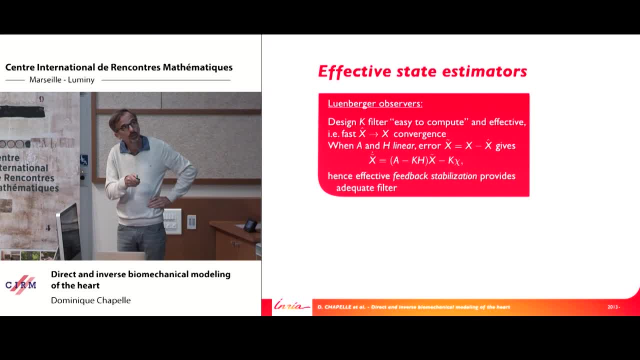 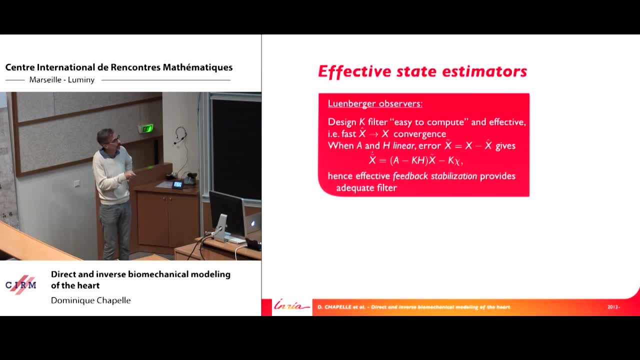 if you have an effective feedback operator for your original system, you can use this to build a filter that will stabilize the error X tilde to zero, which is what you're trying to achieve. Bringing X hat to X means bringing the error to zero. 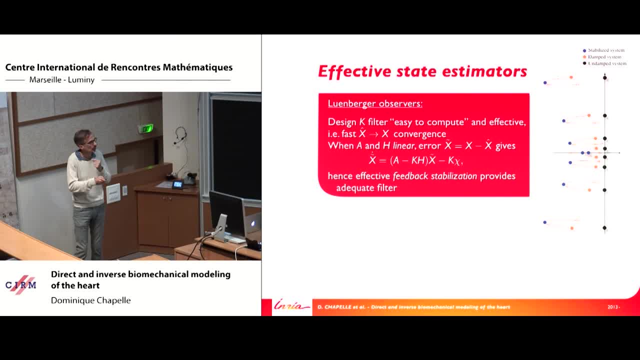 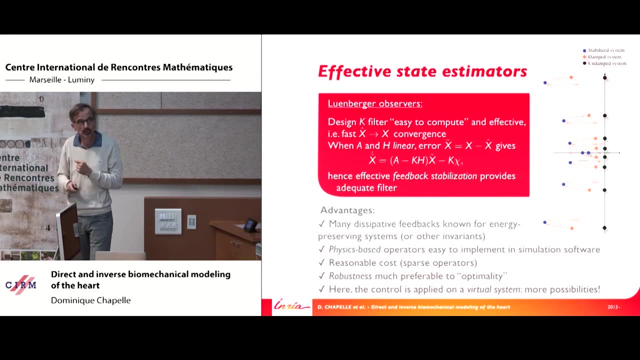 Well, it's a typical problem in automatic control. so what you want is bring the pulse of the system as much as you can to the left-hand side of the plane, and so on. And then the advantage of this strategy compared to Kalman is that, for a wide range of systems, 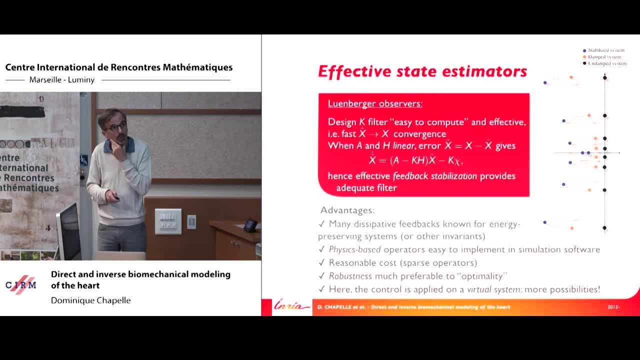 you have many feedbacks that work. actually, Most of them are physics-based, so they're easy to implement, including in the simulation software. Frequently, actually, the operators are already available in the software at a reasonable cost and in a rather robust manner. 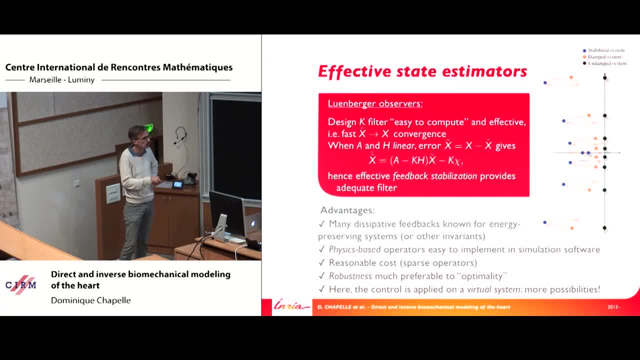 Robustness, in this case for a real system, is much preferable to optimality that would be theoretically provided by a Kalman filtering. Last but not least, the control. the feedback is applied on not a real system but a virtual one. 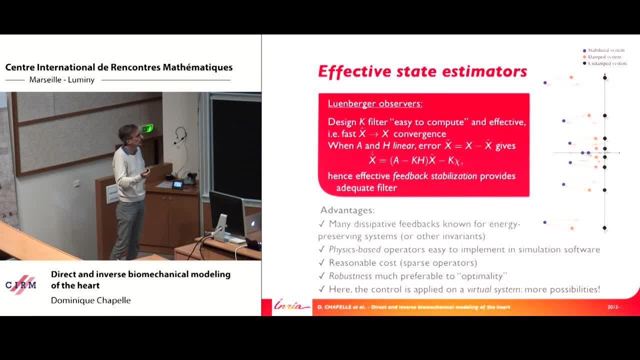 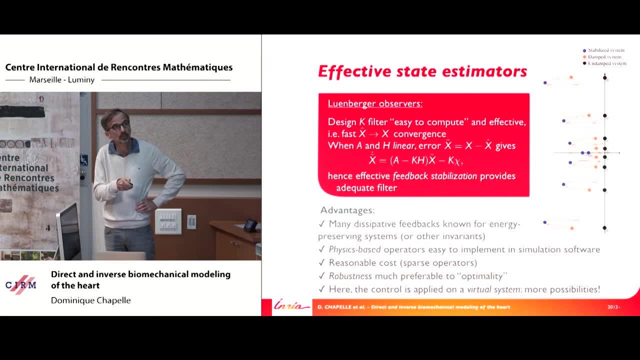 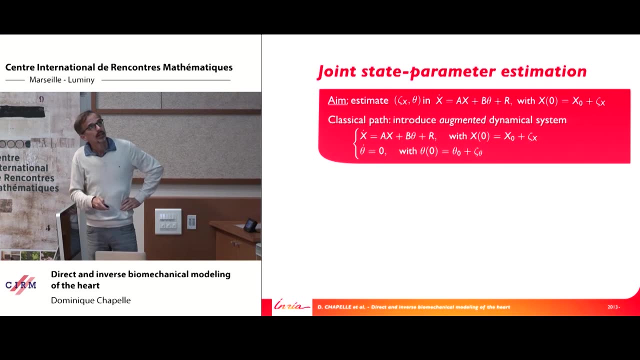 So it means that you can think of a much wider variety of feedbacks. You can extend the dissipative feedbacks that are known for the actual systems. Now, what do you do? This was for state estimation, so this typically is to cope. 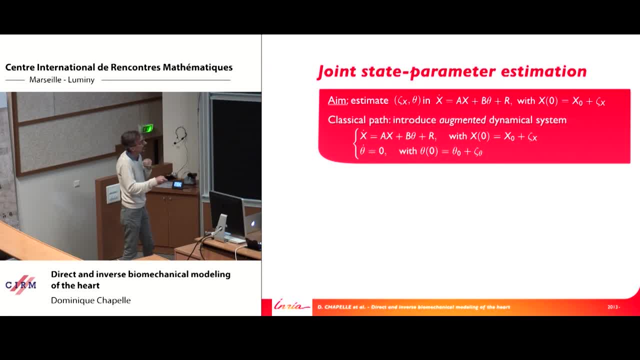 for the initial uncertainty in the initial condition. Now, in general, you want to also estimate parameters. Well, this is the basic principle. What you do is, in the same type of setup, you consider what's called the augmented dynamical system. 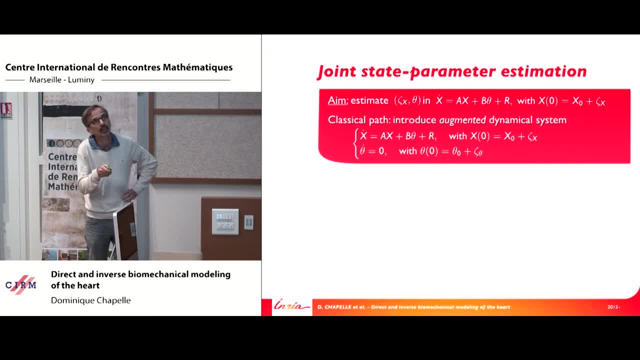 So you have the first equation. We suppose that parameters here enter in a linear manner in the dynamical system. Of course there are extensions to this, And then you introduce the additional equation that describes the parameter that is zero dynamical. Okay, parameters don't move. 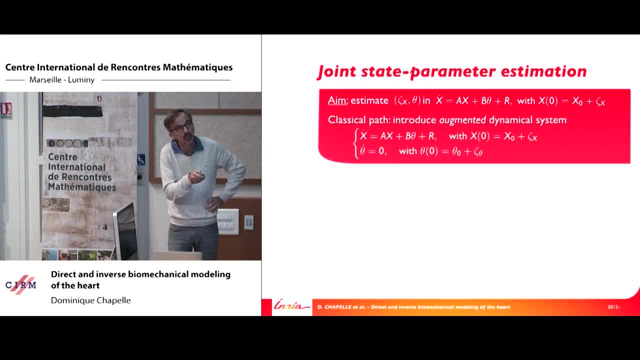 at least in the timescale considered here, And you have uncertainty on the initial condition. So the uncertain parameters turn into uncertainty in initial conditions here And you can apply iterating strategies as before. So for example, Kalman, But Kalman again. 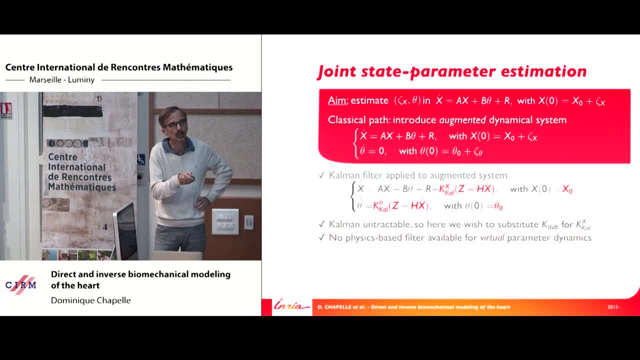 is not tractable for the state part, even though it could be for the parameters. So what we would like. so you have, in this case, two: the Kalman graph, the Kalman gain, could be split into two parts. But what you want is: 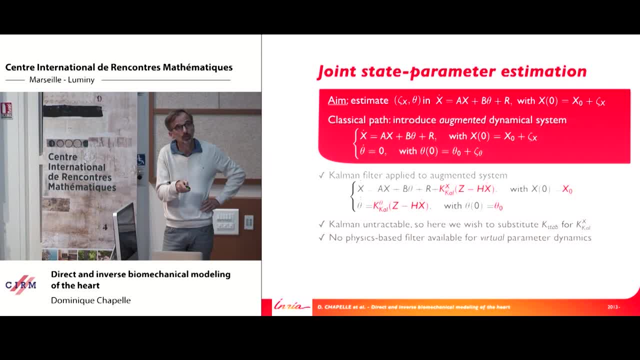 not use Kalman for the state, but substitute this Lohenberger type that we have discussed. The difficulty is that for the parameters, you don't know of Lohenberger strategies that work, because the dynamics is not physical. So what you want here is: 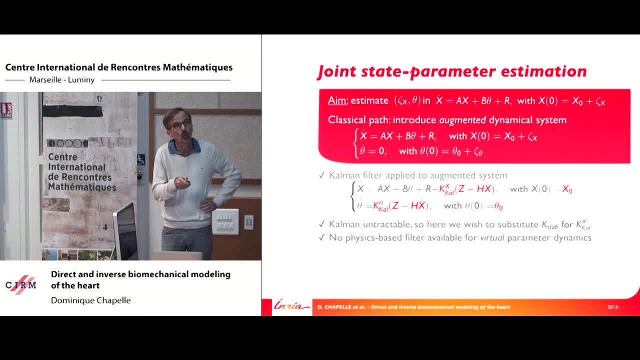 in essence, to retain Kalman filtering while changing to Lohenberger observer here. Well, this is. we show that this is possible And the way you do it. so you use the Lohenberger observer that works in the state equation. 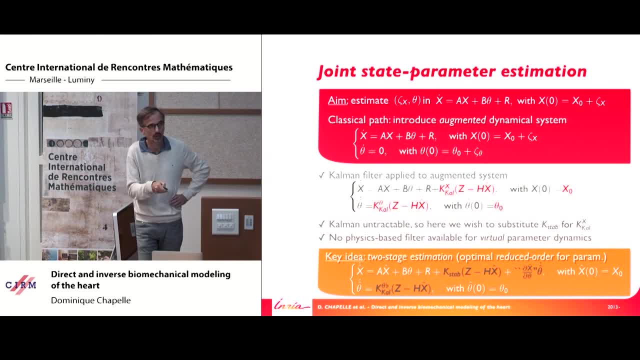 You use the Kalman filter for parameters and then you need to correct the first observer equation by sensitivity of the state with respect to parameters, with no virtually little additional computational cost here, And we showed that this is actually effective in a series of papers. 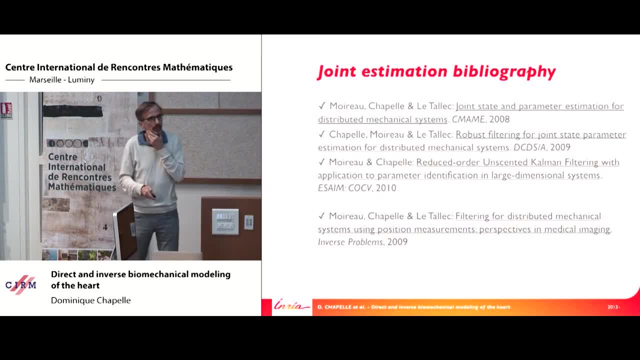 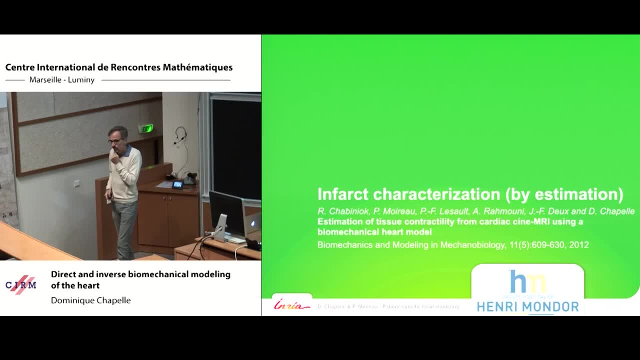 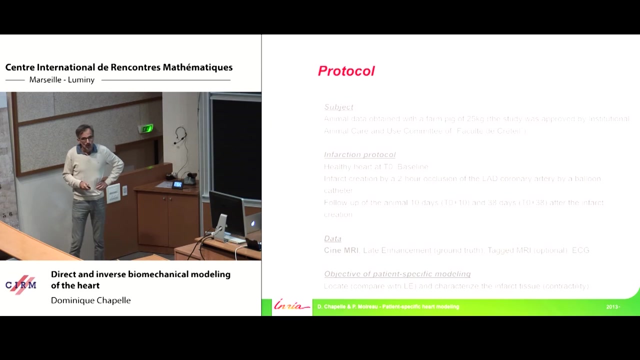 Now, quickly, in the remaining time, I will show you some application of this, using medical imaging to characterize an infarct by estimation. So this is again a collaboration with a hospital, in this case in Créteil. We used some, again some animal data. 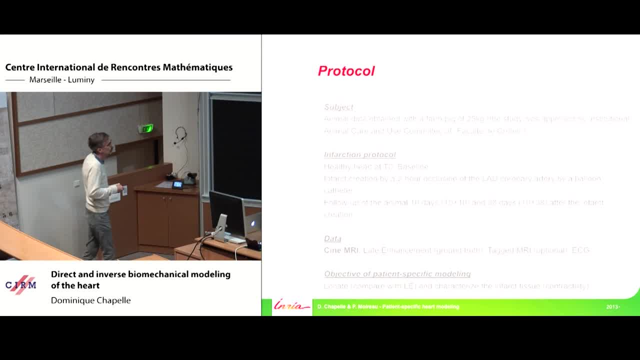 obtained on a pig on which an infarct was actually created. So the idea here is, by occluding the coronary artery of the pig, to control the extent and location of the infarct, And this will be used for validation purposes of the whole estimation process. 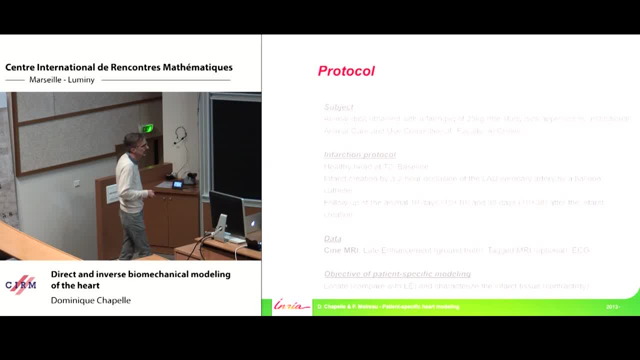 We have, of course, as data, we have a lot of imaging pressures and so on, And the idea will be to use this modeling and estimation chain to characterize, that is, locate and estimate, the parameters regarding the infarcted tissue. 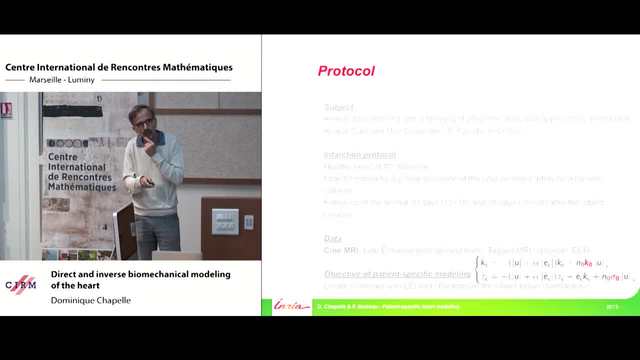 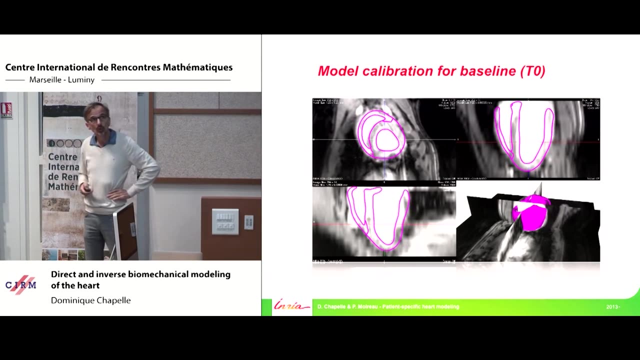 So what we want in this case is to estimate the contractility parameters, that are, these quantities in the active modeling parts of the equation. Here is a calibration- again model against MR sequences in baseline. So that is before the infarct was actually created. 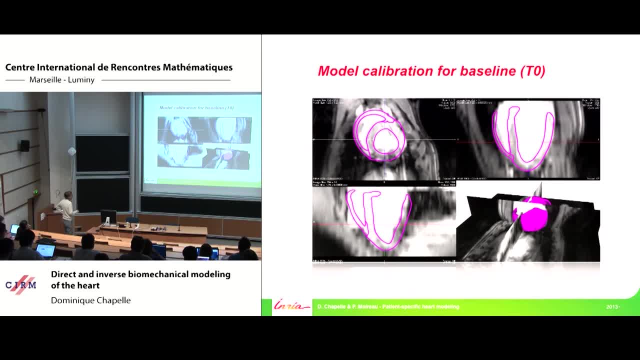 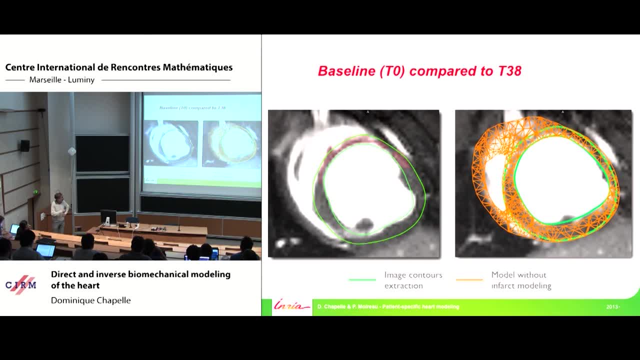 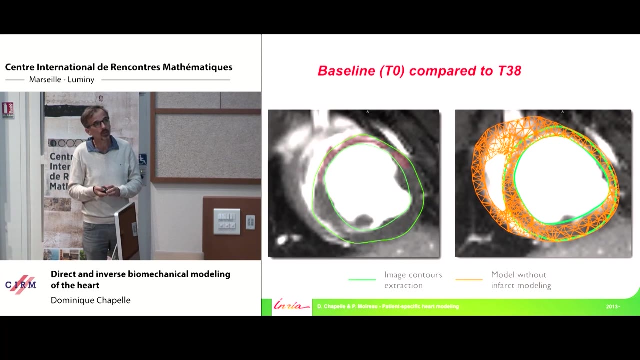 So again, a nice equation of the model and the images, And now this shows you the type of infarct of data that will be used in the estimation framework to perform this whole estimation strategy that I outlined in the previous slides. So what we used are: 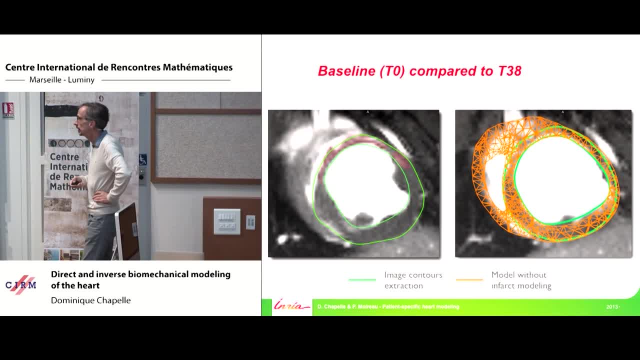 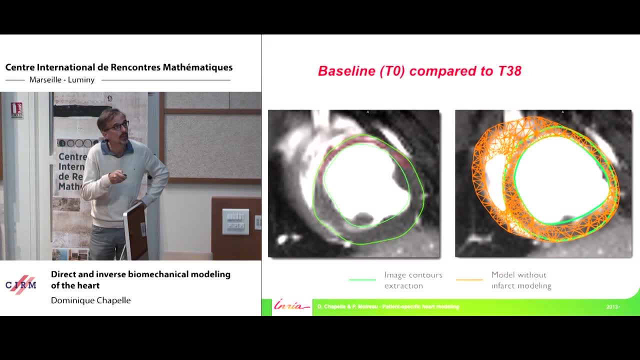 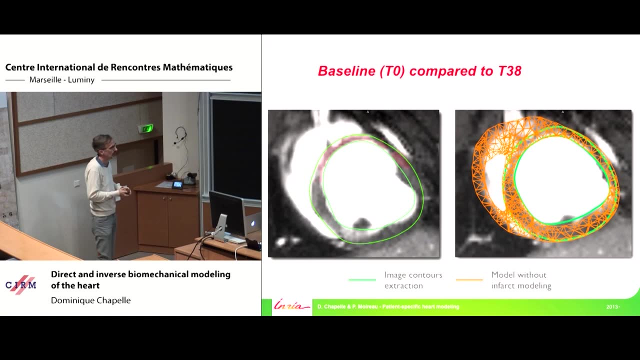 segmented surfaces of one single ventricle, in this case the left, the main ventricle. What you vaguely can see in orangish over here are the parts that correspond to the infarcts that again are known both from the controlled protocol and here also from one. 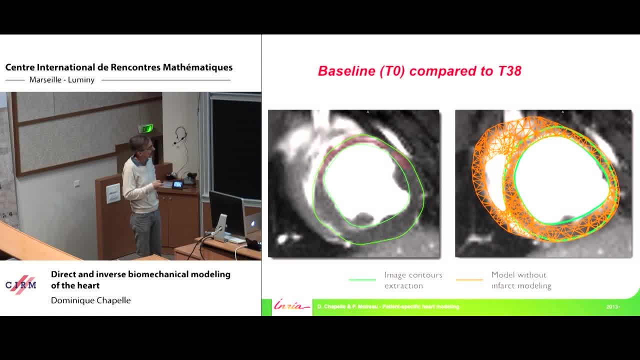 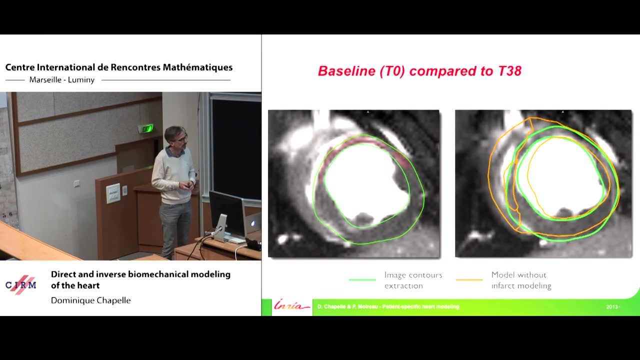 specific modality of imaging. So we have a control. Now what you see here is the healthy model, So the model that was calibrated with respect to the baseline data against the data here in the infarcted heart 38 days after the infarct. 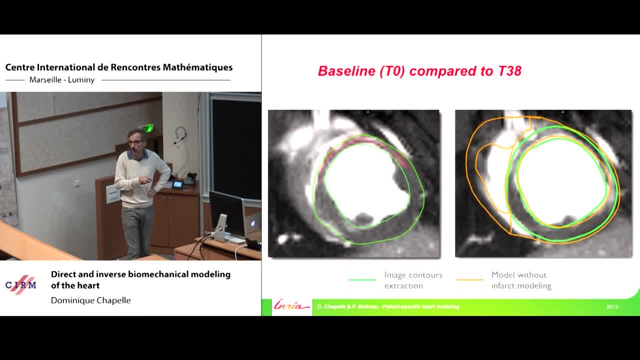 was created. Of course, the healthy model doesn't know about the infarct and it contracts much more strongly than the actual heart at this stage. So you have this pretty big discrepancy and this is what's going to be used in the sequential data estimation strategy. 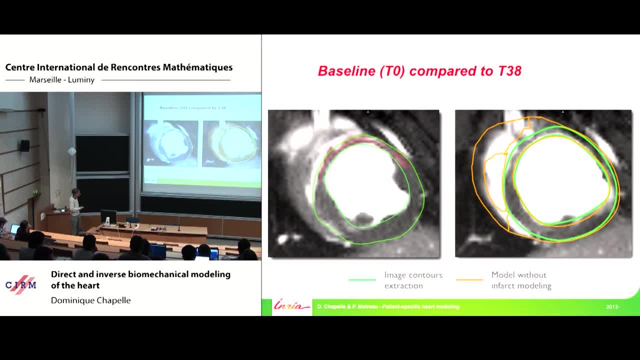 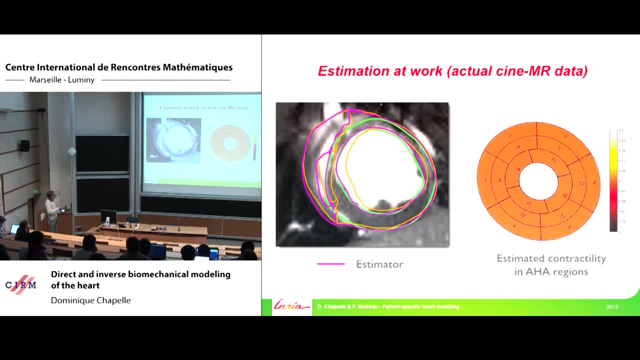 to correct the dynamics and estimate parameters at the same time. So here what you have is the corrected the observer system in magenta. As you can see, it's quite close to the data. It doesn't have to be exactly coinciding with the data. 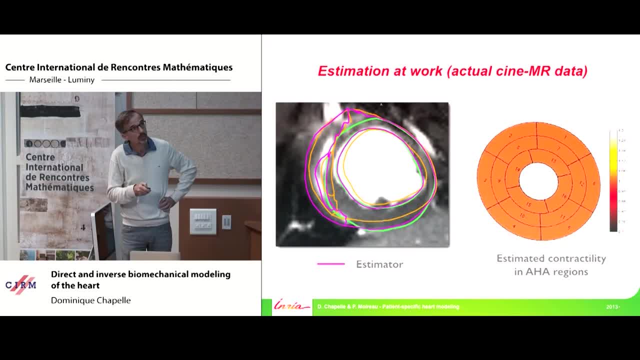 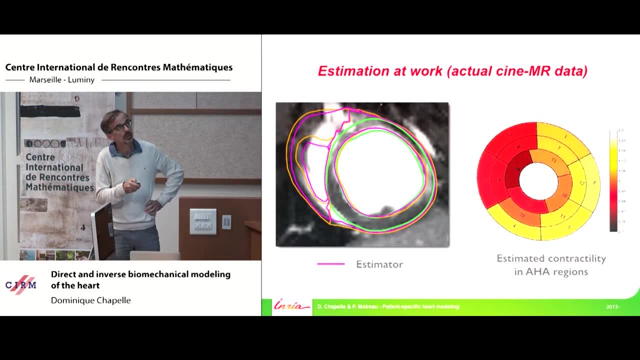 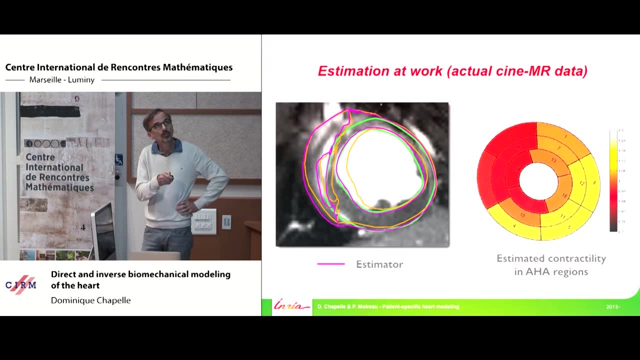 It's just a correction, But it's very close to the actual walls. And then the orange was the heart before infarct. So you can see it's a big difference. And in the same time we estimate one quantity in various regions of the heart. 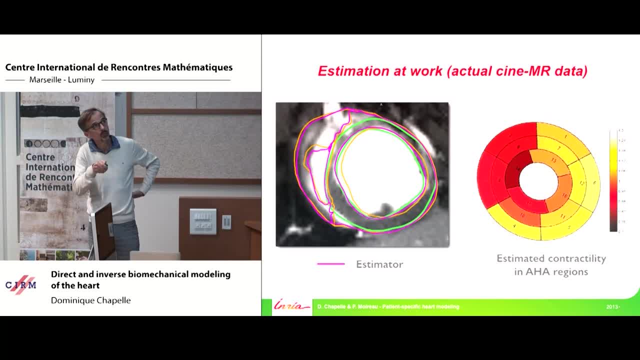 So this is a view from the top of the ventricle. This would sit on this part, And dark means low contractility, Light, high contractility. As you can see, the dark contractility really represents the part where the infarct. 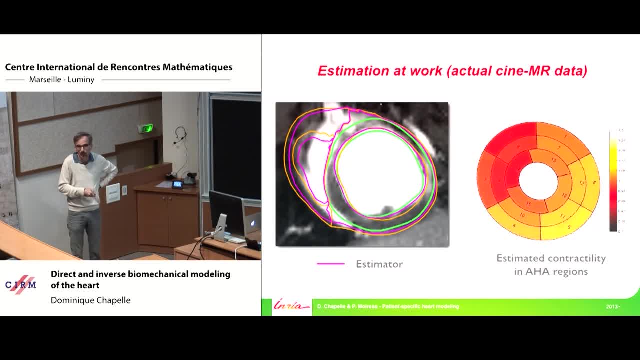 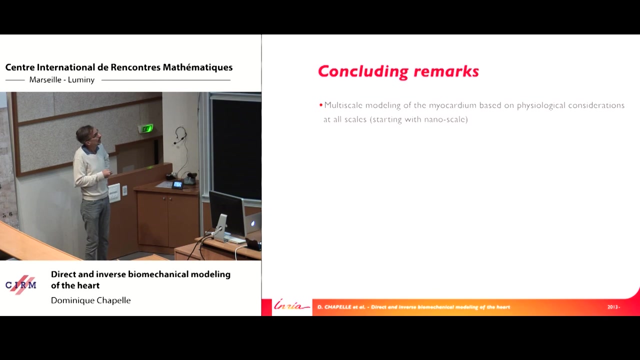 was actually created. So of course we don't have any ground truth in this case other than this control information. but it's quite a nice validation of this estimation setup in a real data clinical setup. So, concluding remarks, I summarized the type of multiscale modeling. 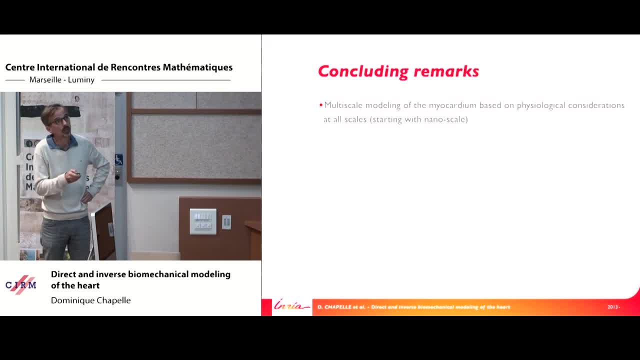 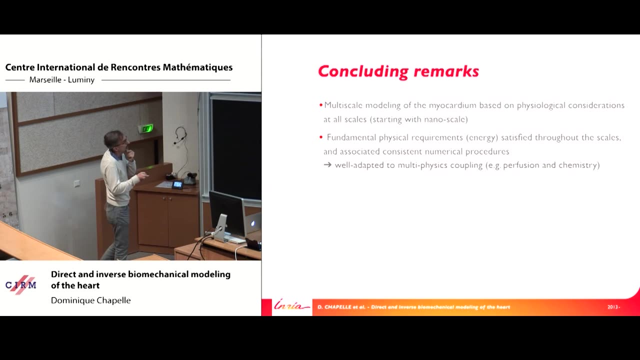 that can be performed to represent the myocardium, based on actual physical and physiological considerations. at all scales, Starting with the nanoscale of the actin-myosin bridges, We carried fundamental physical requirements, in particular energy balance, all the way throughout the scales. 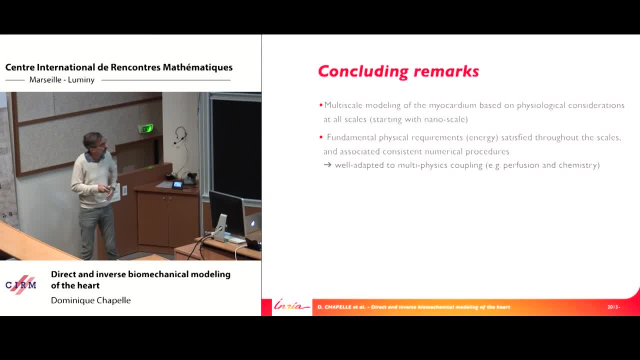 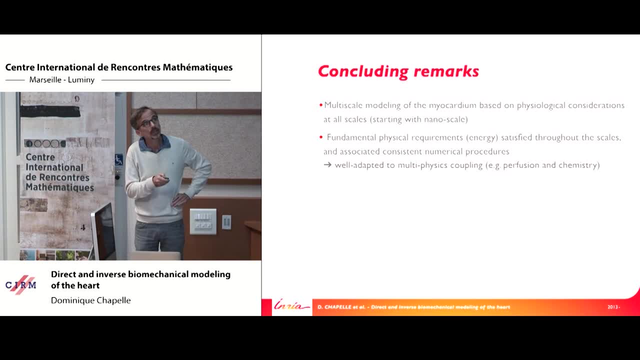 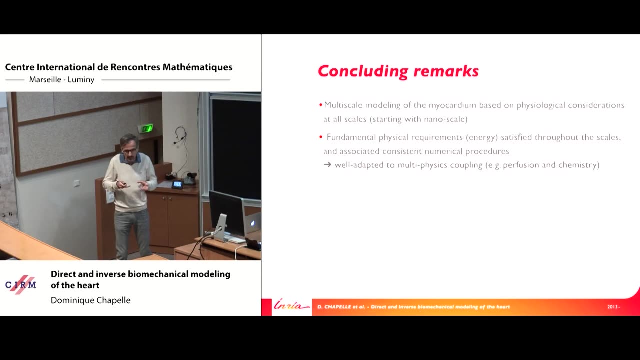 And this is actually also true for the numerical procedures that we design. So these numerical procedures satisfy the energy balances. This, of course, is well adapted to multi-physics coupling, because when you want to couple to other phenomena, chemistry, fluid flows within the muscles. 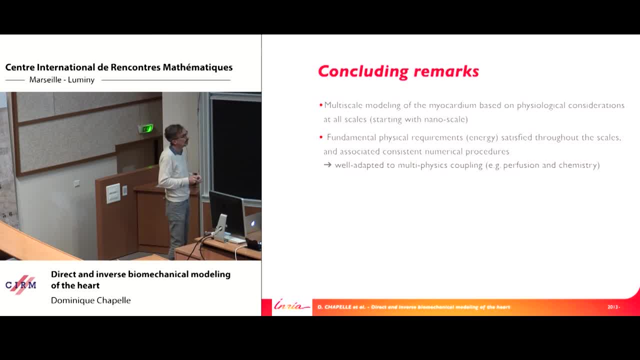 that is so-called blood perfusion. All this will mean that you will be able to formulate the coupling in an energy consistent manner If you start by components that satisfy these balances. We have already some substantial experimental and clinical validation, as I showed, And I also covered. 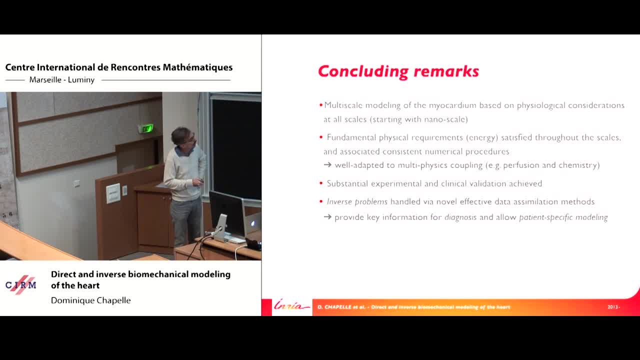 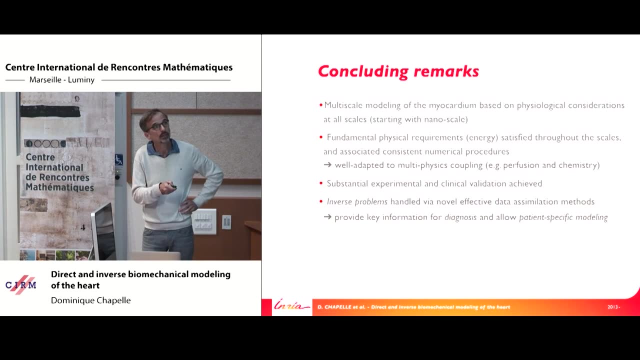 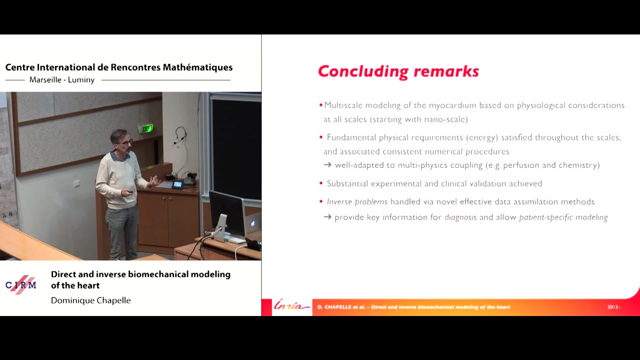 the inverse problem that you need to solve in this case And showing that in our team, we focused on some novel types of data estimation methods that we designed, And this provides, of course, key information for a diagnosis, because once you estimate some actual parameter values of interest for medical purposes- 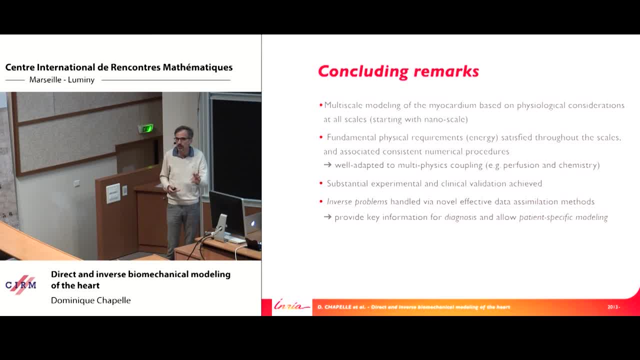 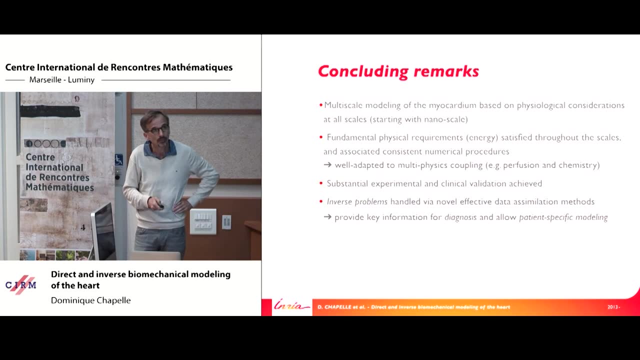 for example, this contractivity value here has a meaning for a cardiologist, And this parameter cannot be measured in any other way in practice. So here you provide something that's very important for diagnosis And then, once you have adapted your model to the patient, 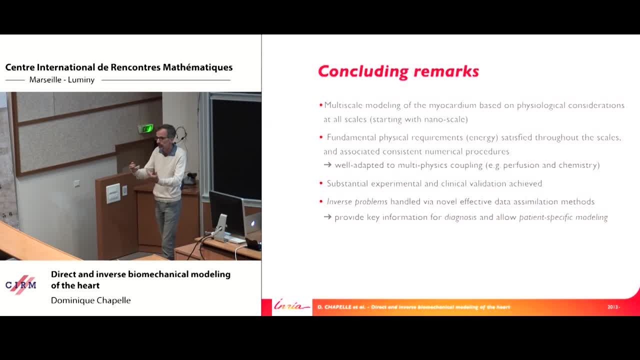 you can carry out the program of patient specific modeling, That is, you can use the model to predict the future of the system. that is typically the outcome of therapeutic strategies, as I showed in the first place. Again, if you want to have a predictive model, you need to adapt it. 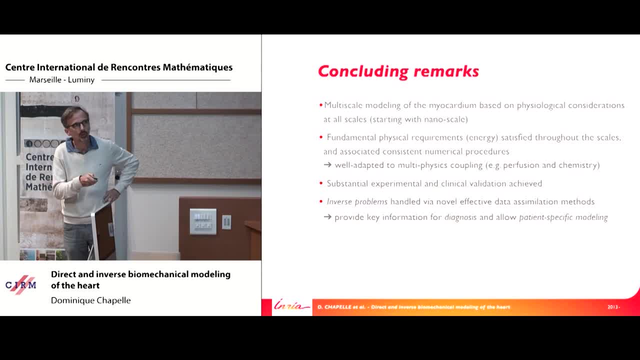 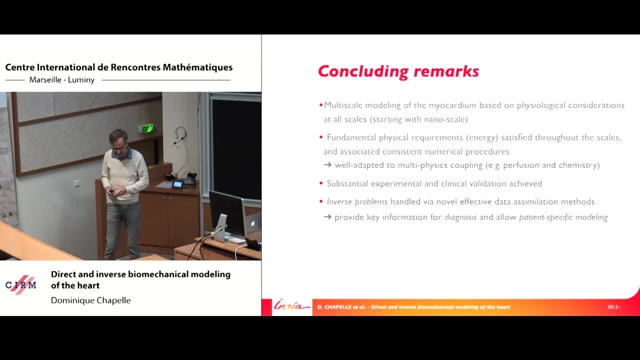 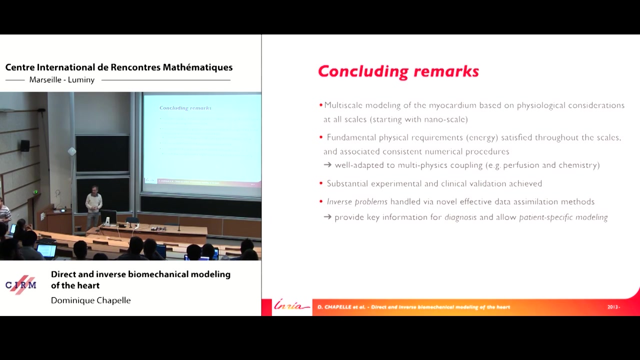 to a given case. So here the inverse problems have two benefits: Diagnosis, when you estimate, and then prognosis, when you use the predictive nature of the models. This is the end of my talk. Thank you very much for your attention. Thank you, It's just a very naive question. 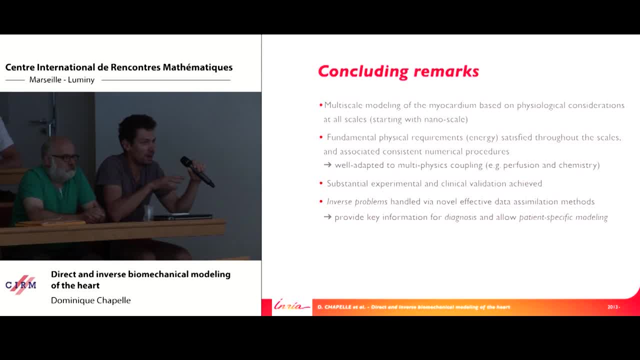 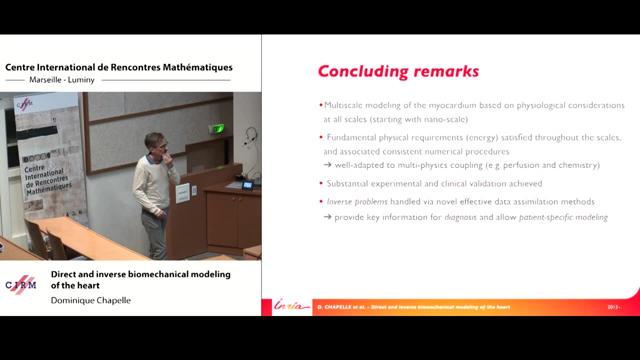 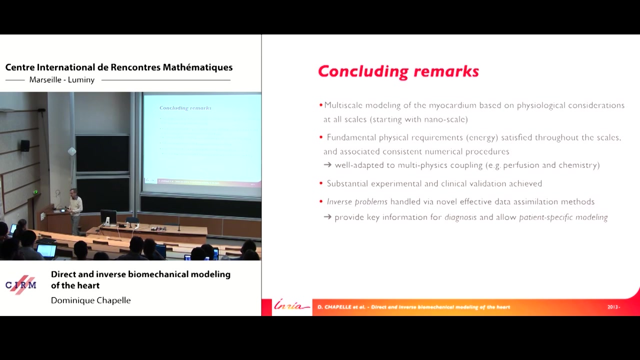 concerning the last part of your talk, Do you have some issues of observability of the state when you estimate the parameters and the initial state? so it's in practice, I mean Well, of course, this is a very complex problem. It's a major issue. 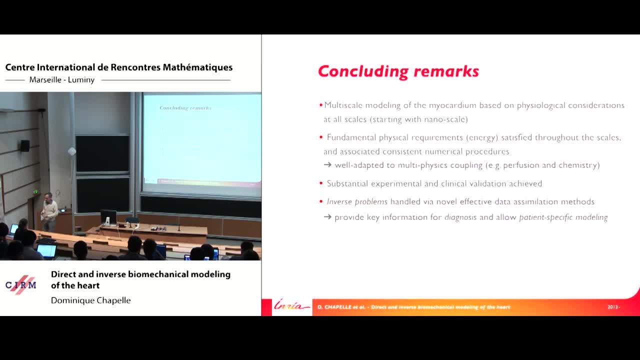 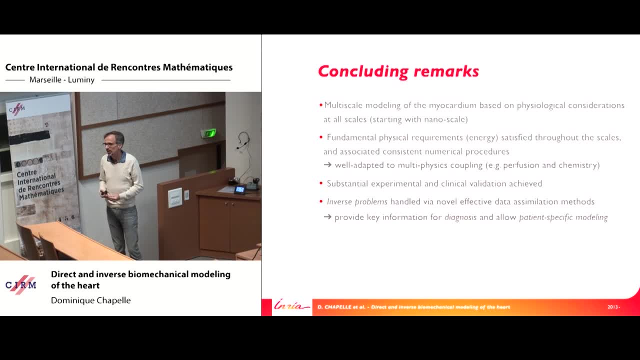 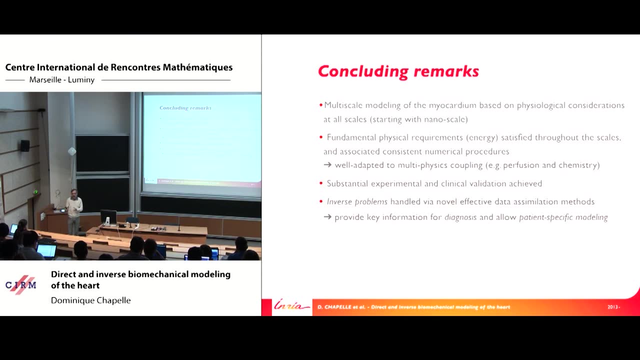 in estimation and inverse problems, So it's not something that you can answer in a unique manner In general. so, as you mentioned, it needs to be addressed, if not only in practice, but it needs to be addressed by looking at a given type of setup, that is, a model. 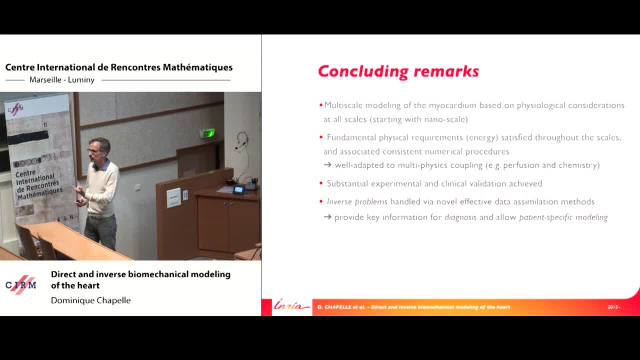 that needs to be estimated versus the data that you have at hand to estimate the model. In our case, the problem of observability is mainly an issue for identification purposes, That is, it's more an issue for identifying estimating parameters than for estimating the states. 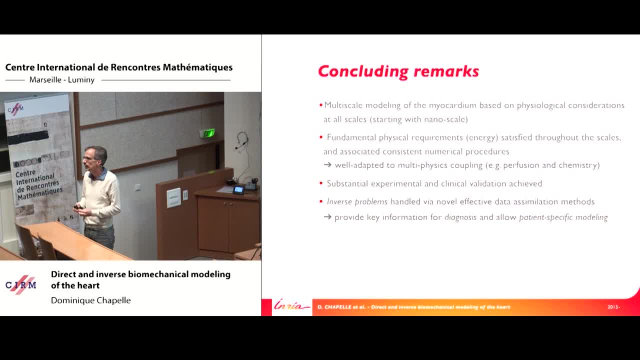 Medical images are very rich, as you can see, So it means that it's, in practice, highly identifiable in respect to the state, Whereas what you can see in terms of parameters of course depends on not only the kinetics but also the richness of the description in the model that you have. 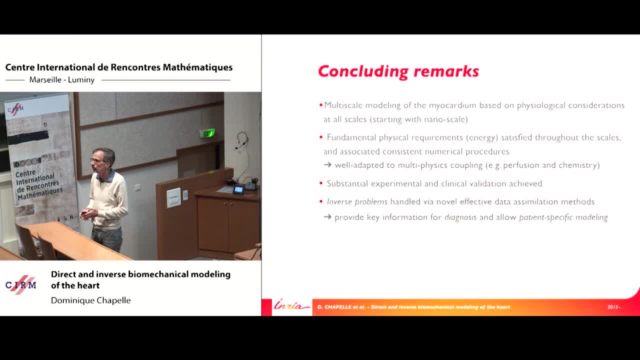 So if you want to estimate large numbers of parameters, which means that you have, for example, complex pathologies with multiple components of the system that are affected- then you may get into trouble in terms of estimation. The good news: with the type of strategies that we have. 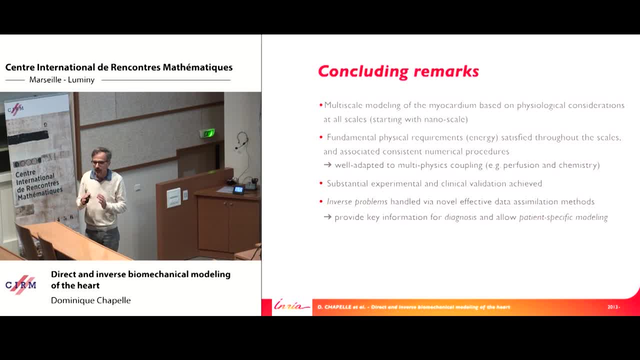 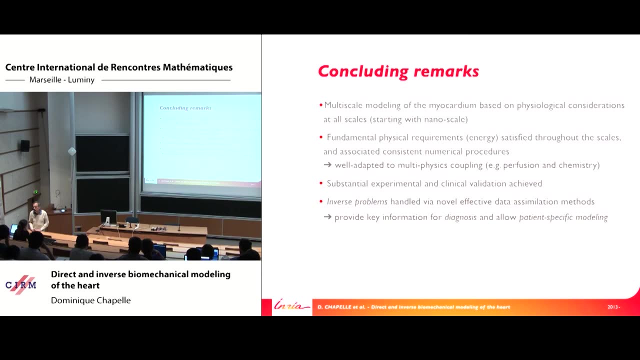 so sequential strategies is that in the end, you not only have an estimate of the quantity itself, but also you have an estimate of the error that you perform. This is hidden in this covariance operator that you are actually computing also, You see, so it's a. 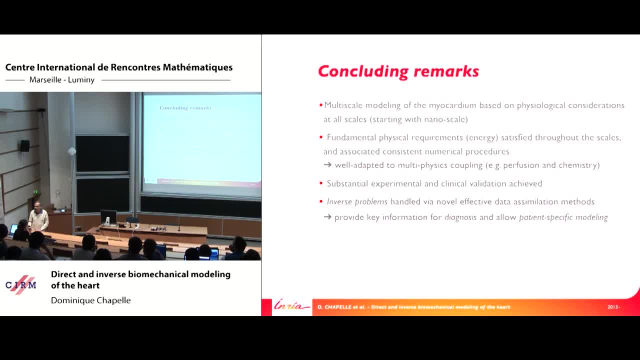 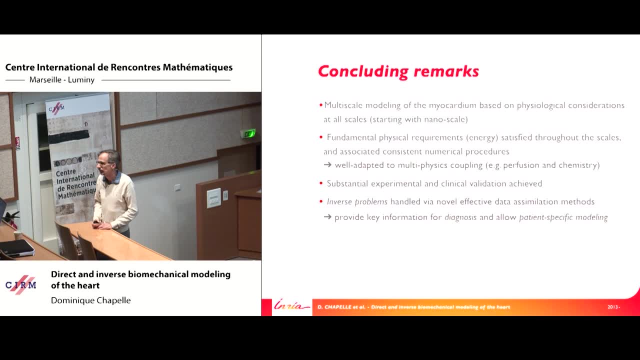 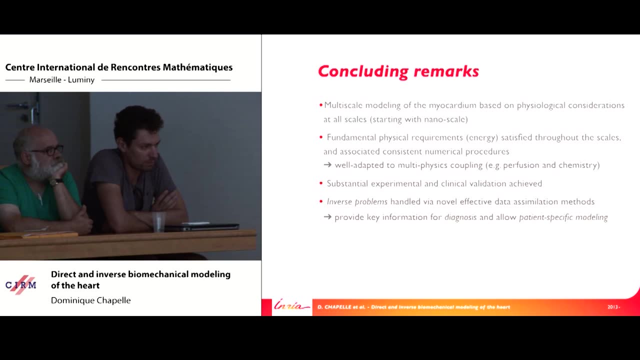 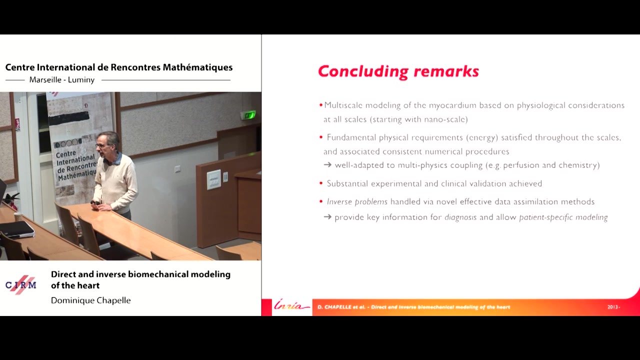 you have an answer, but you also have a level of confidence in the answer, in the estimation, And then there are lots of additional considerations that you can include a priori to assess the identifiability character of the system, And for this you should. the expert is right here. 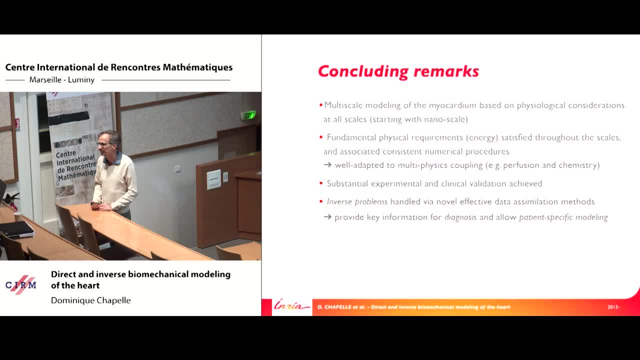 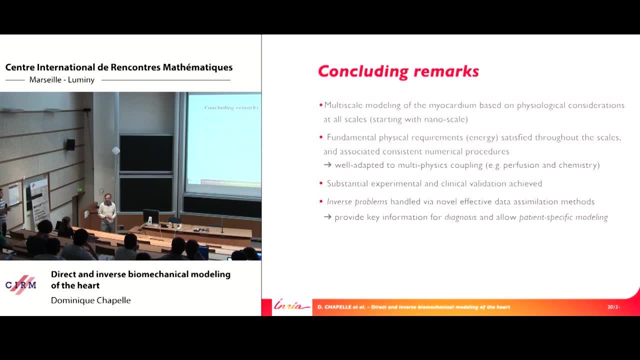 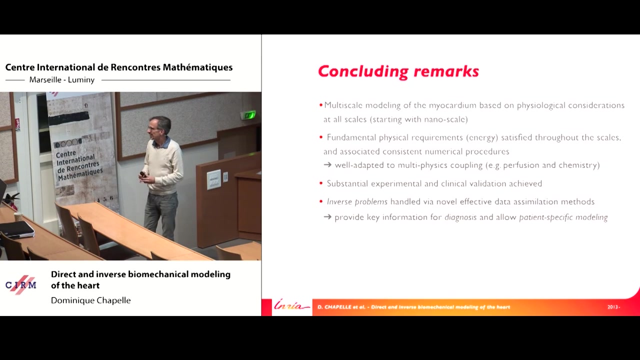 so you can ask him afterwards Other questions, Maybe a short one about the HPC challenges that you have to deal with for this kind of big simulations. Well, it's a tricky question. He's doing it deliberately In our team. we are not. 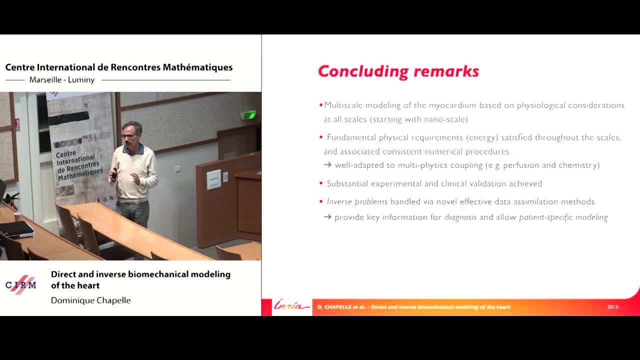 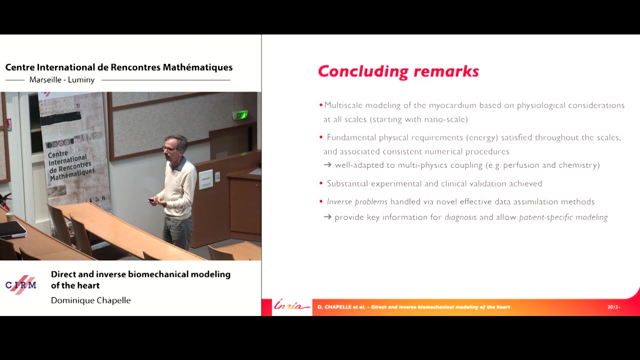 HPC focused. So we know that HPC is highly technical. We cannot cover everything. You have seen that already. we cover quite a large spectrum of topics. Of course these are highly non-linear multi-physics model, So we always limited by the computing time.